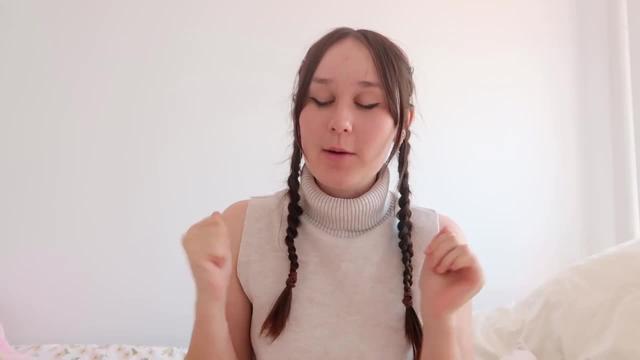 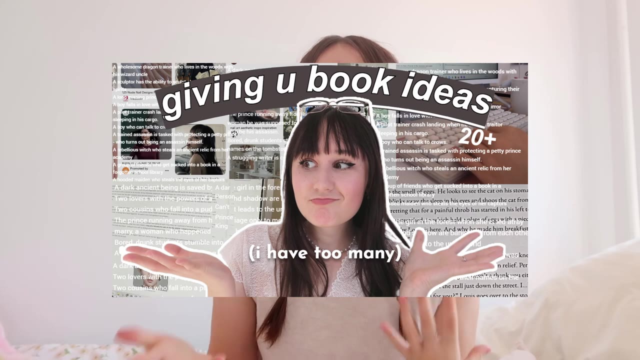 Hey, Rally Besties, welcome back to my channel. I hope you're well. Today I'm really excited to just talk about some book ideas, My other video. this video did so well and a lot of you guys actually really did enjoy hearing some random ideas that I have for books. and yeah, if you guys don't have 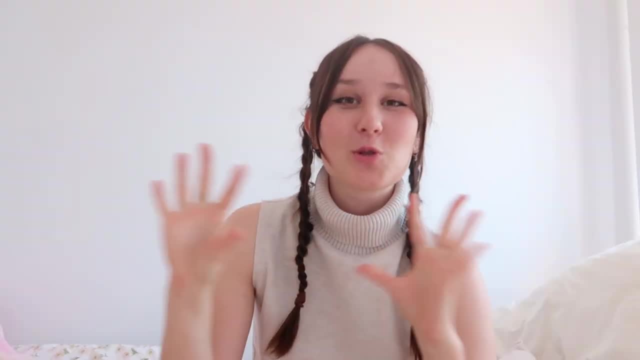 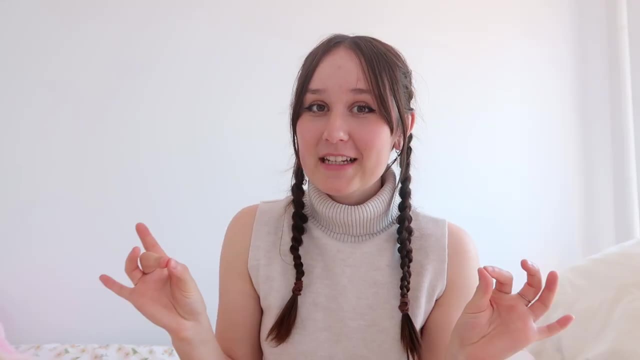 any book ideas. I have so many for you. I have so many, so I'm so excited to get into another 20 book ideas which you can use to start your own novel. I do want to give a huge shout out to Milanote for sponsoring this video. Thank you so much, Milanote. If you guys don't know, Milanote- 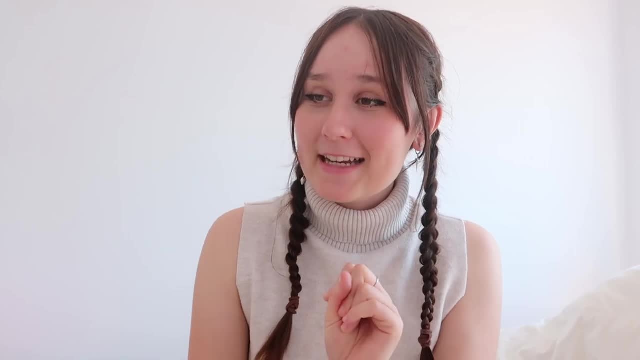 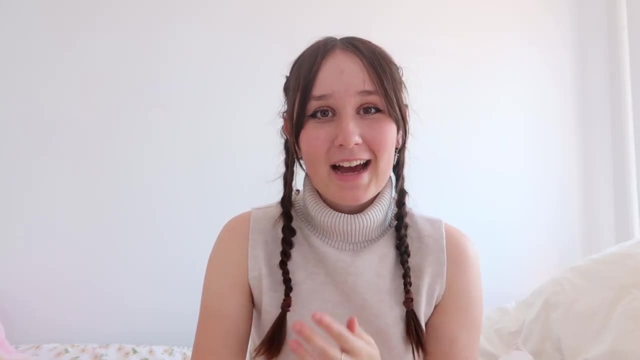 they are amazing. Especially if you're going to brainstorm some of these book ideas, you need to check out Milanote. Milanote is a free online space for you to brainstorm anything you like If you're creative and you love to brainstorm, love to plan, love to create little boards for. 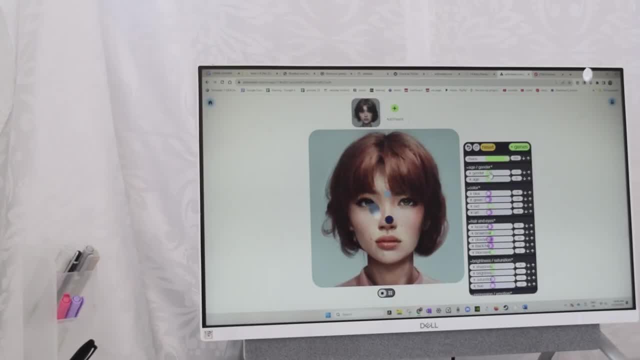 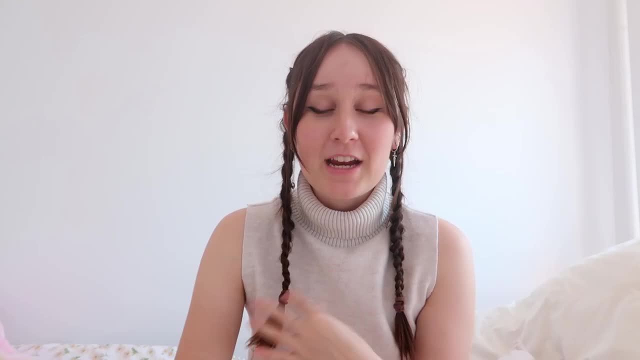 your books, for your projects, for your schoolwork- literally anything. Milanote has an amazing space for you. I'm currently using Milanote for my book ideas. If you're interested in learning more about to create one of my novels and to brainstorm one of my new projects called Project Samson, and I think 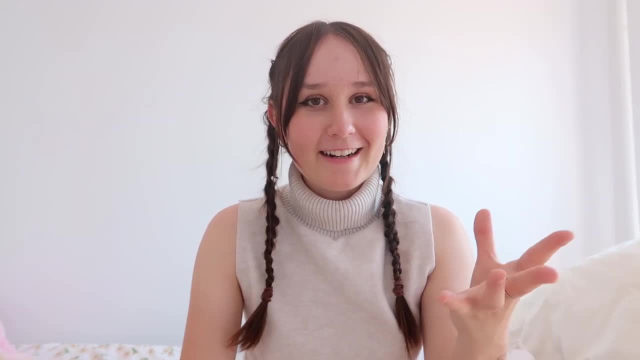 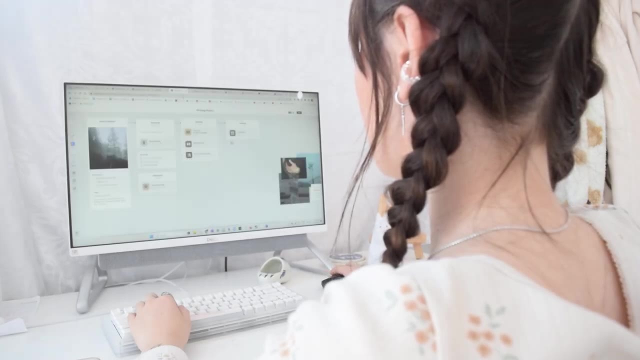 it's really helpful because if you guys are creative- I guess you're a writer- you know how messy it is, especially starting a new project. So Milanote is an amazing and free space- yes, Milanote is actually free, by the way, to brainstorm your ideas, Something that I always say in all my videos. 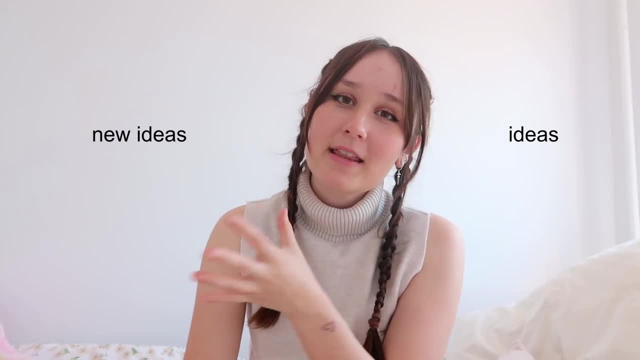 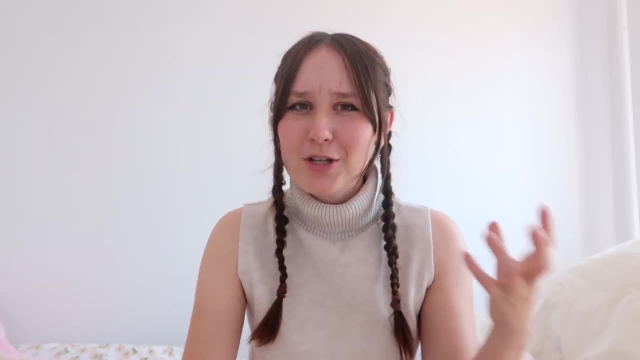 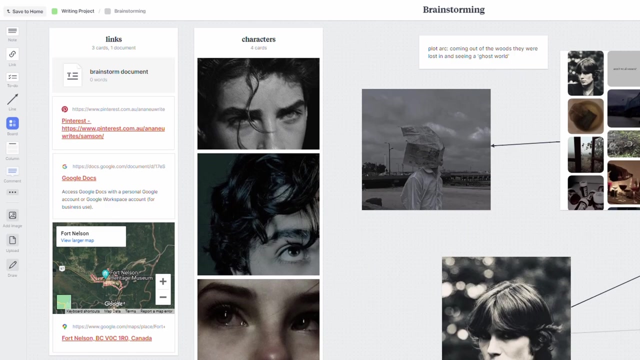 is that ideas inspire new ideas. So the way that Milanote works is they create amazing boards which can draw a lot of different types of media together, So you can create Pinterest boards. on there, you can link playlists, music, YouTube videos, images and characters and plot templates. 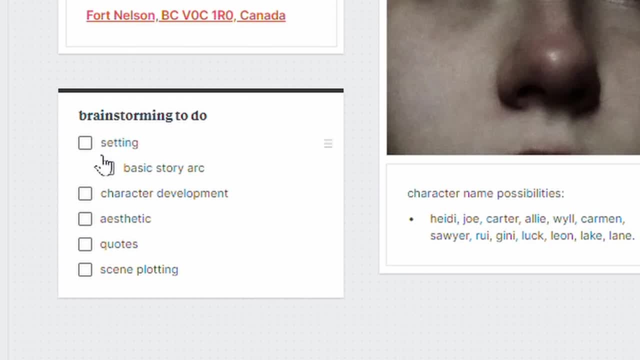 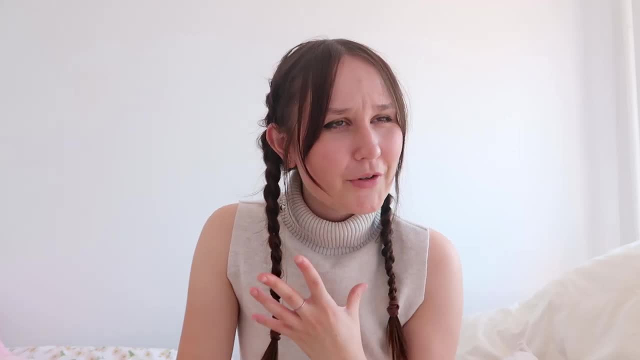 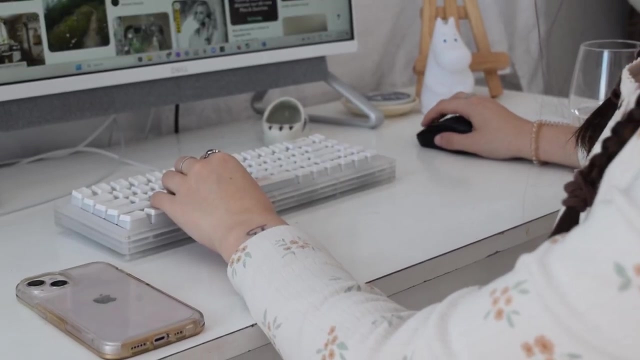 It's such an amazing space and, of course, Milanote helps you organize all these ideas and all these brainstorm spaces in a way that's actually really personalizable. How do you say that You can personalize your stuff basically, So, whether that be a script, a new novel, a chapter, a blog or a creative project for school like you can use? 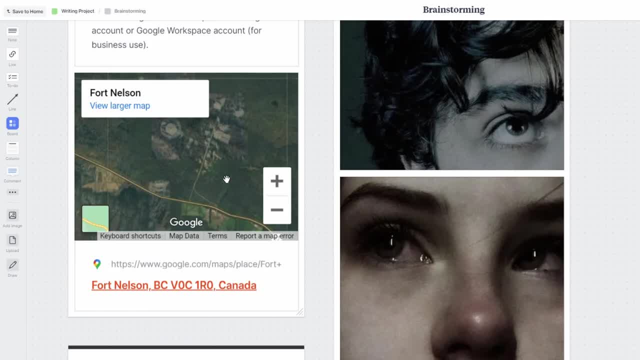 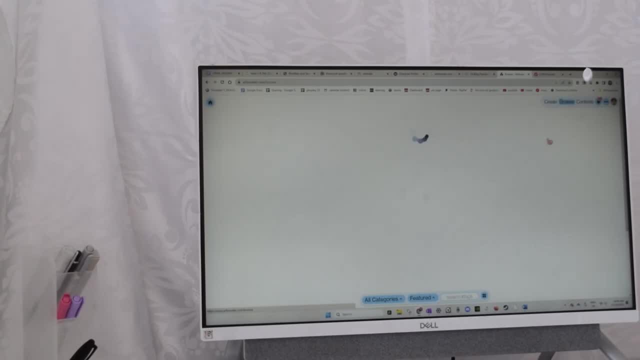 Milanote for anything And, of course, the one thing that I love most about Milanote is its flexibility. I use Milanote on all my different devices and, since it's online, it also saves to the cloud, so you will not be missing or deleting or accidentally coming back to your project and 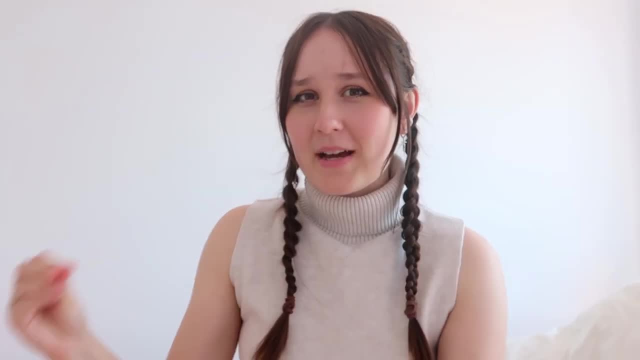 seeing everything gone. Milanote takes care of that. And what's even better is that if you guys are having trouble, you can use Milanote to do that. So if you guys are having trouble, you can use Milanote to do that. So if you guys are having trouble, you can use Milanote coming up with 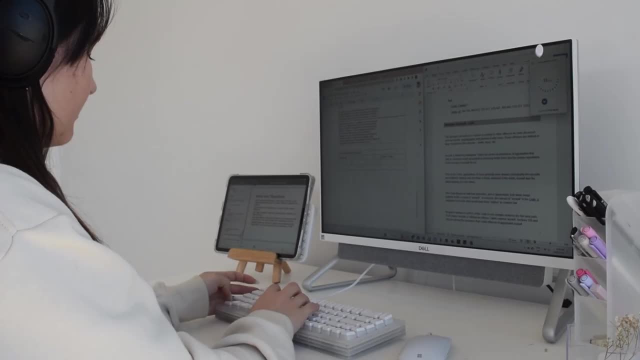 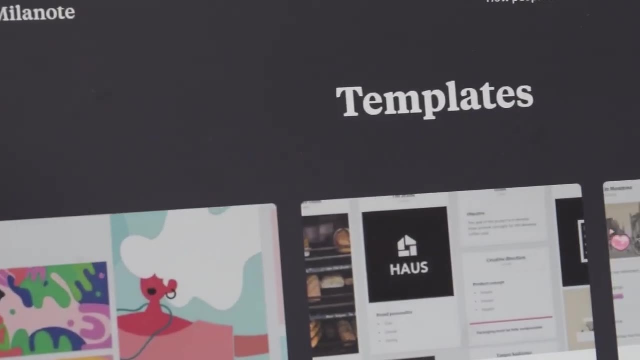 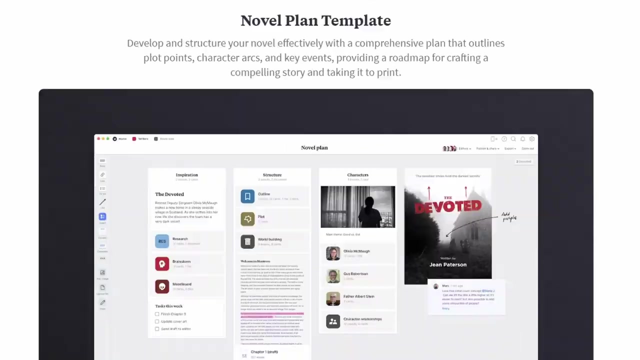 new templates, or you kind of just need a more guided sort of space to really bring forth your creativity and your ideas. Milanote has over a hundred amazing in-built templates that are available to you for free. You can share your boards with your friends and colleagues to and gather inspiring feedback in real time. I also thought. 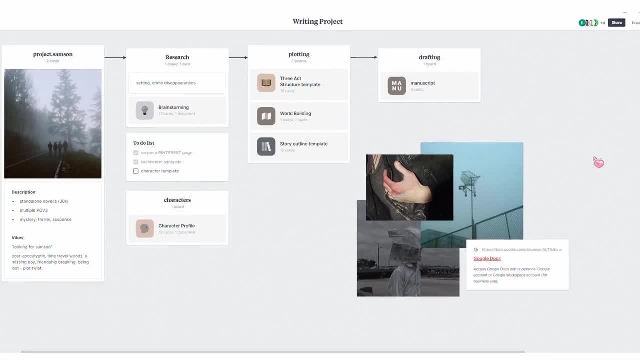 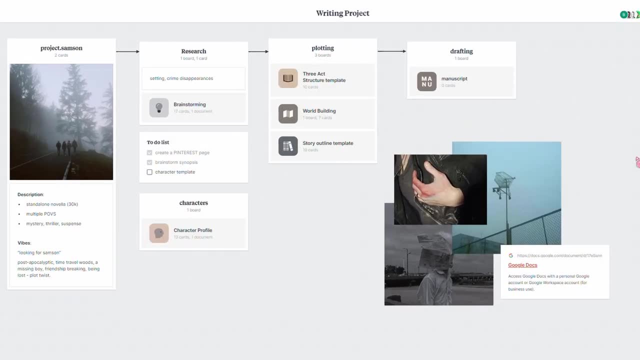 it would be a cool idea just to kind of give you a little bit of a tour of my Milanote, just to show you how cool it is. so if you do get an idea from this video, you can see how you can use, yeah, millinote to brainstorm your amazing idea here. i have project samson, i have all these. 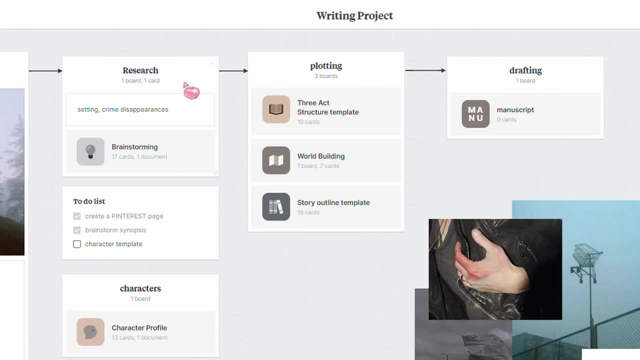 different boards. i have research over here which is kind of all about brainstorming and thinking about your book and, you know, using sort of real settings or real people to inspire your story. and then i have a plotting over here and this is, like all the plotting stuff, um, very loose plotting like 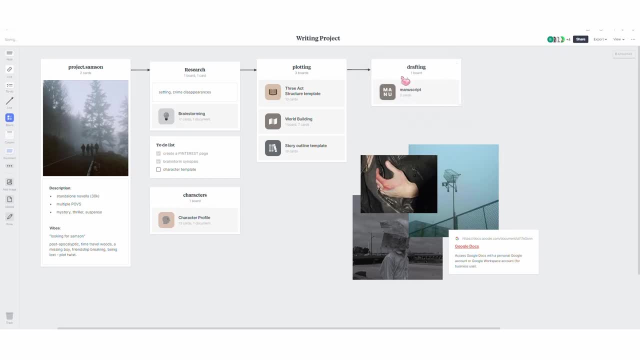 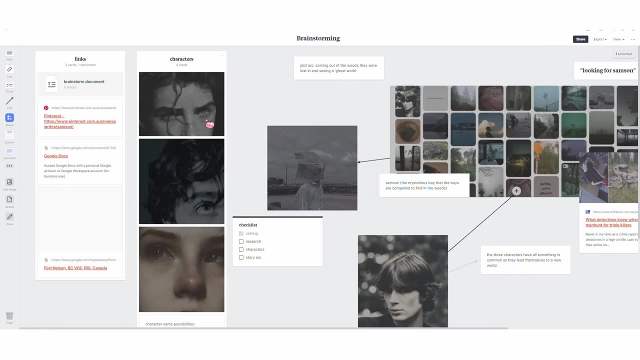 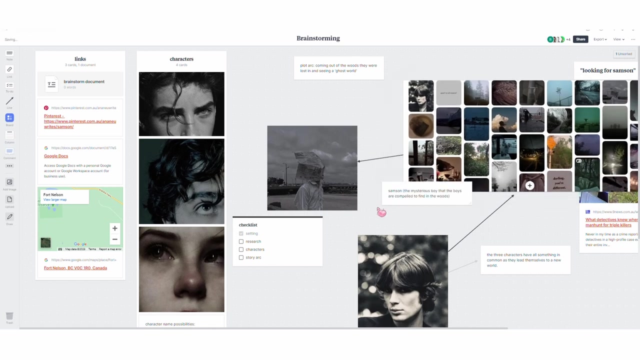 the three act structure template, world bullying etc. and a drafting um little board over here which i have for my manuscript page. my favorite page is actually my brainstorming page over here which you guys have probably seen in some of the previews, but i love how like interactive this is. 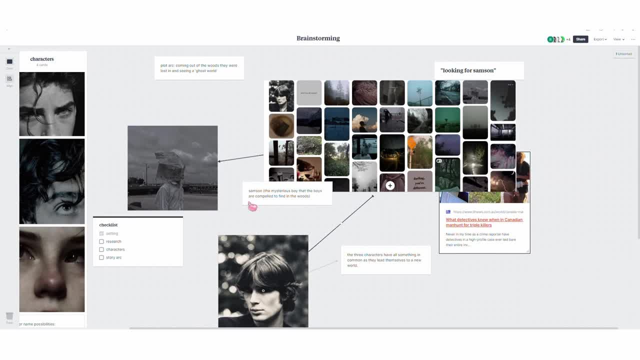 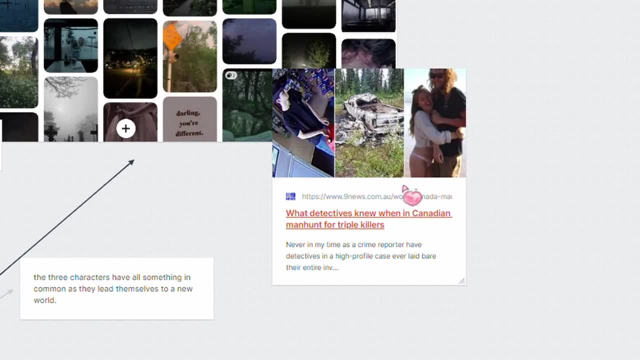 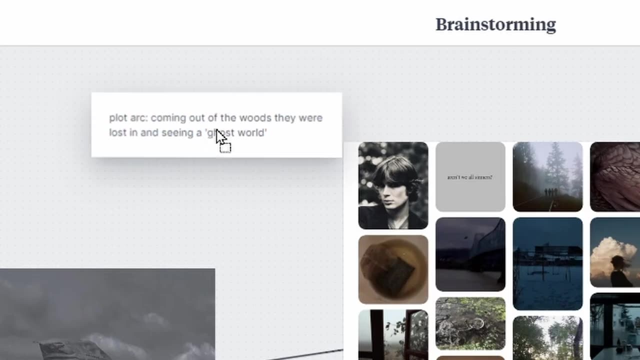 and how you can just, yeah, really, um, see how things work together. um, as you can see, here i actually have like a news story where, yeah, it can kind of actually be inspired by, yeah, a literal news story for this project. looking for samson, i have a couple of little. 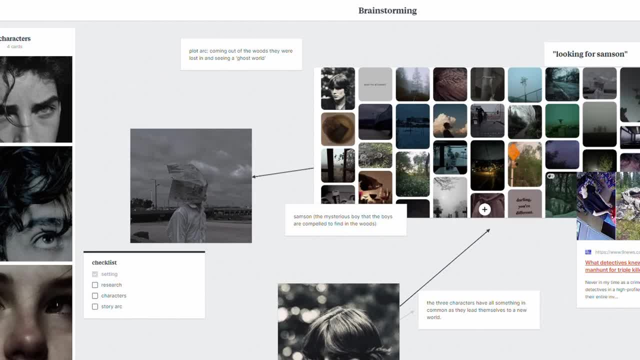 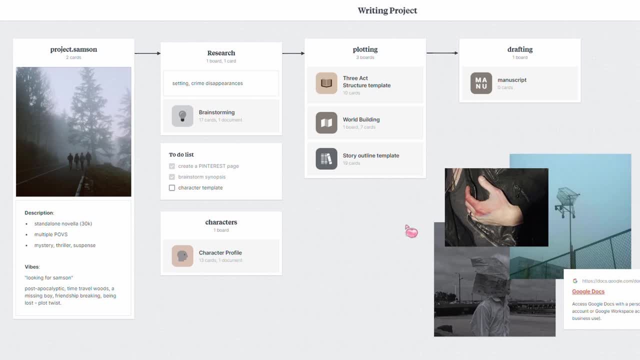 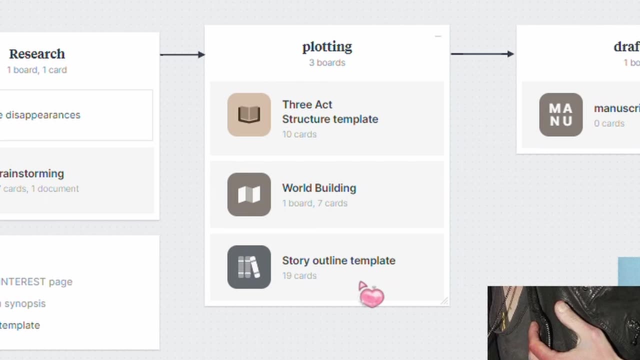 ideas in these bubbles and, oh, it's just such an amazing, fun process brainstorming. i adore it. i wanted to show you a bit of a plotting page because i have been using millinote for a while and this page literally has saved me so much. it is the story outline template. i remember like going to this template and actually 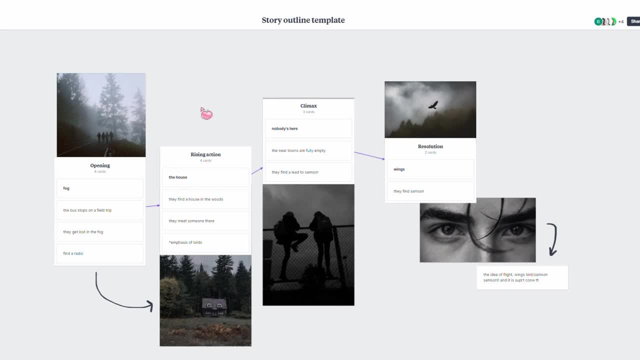 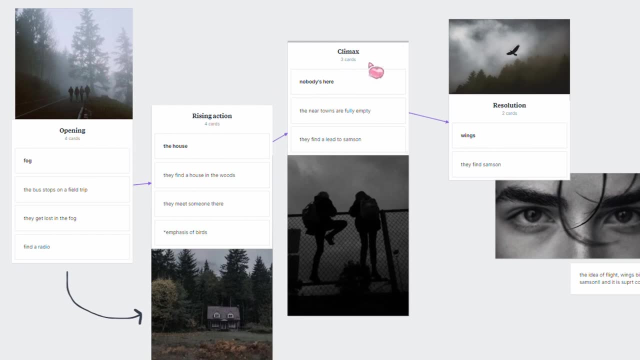 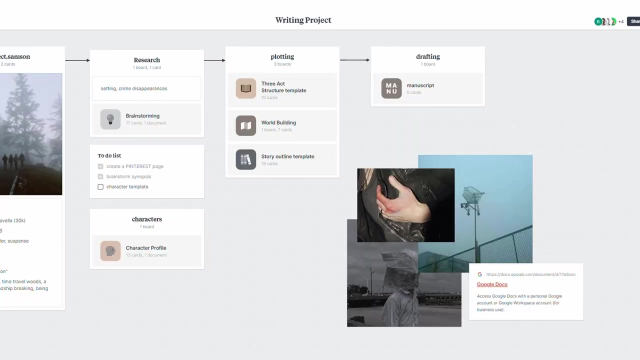 like brainstorming project cz, one of my really old projects. um yeah, and this is what it looks like. it's literally amazing and this is the best. like i hate plotting, but millinote makes it so easy because, as you guys can see, i have the opening, rising action, climax, and then i can go forth and 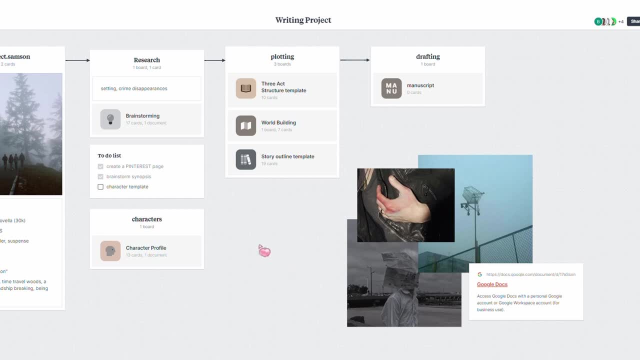 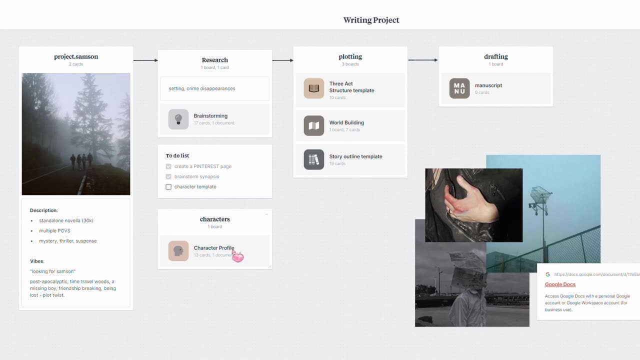 write my zero draft for this book. i actually want to show you guys one more page, because i have a lot of characters, because i'm obsessed with personalizing and creating templates like this. here i have a character profile and this is one of my characters from project samson. 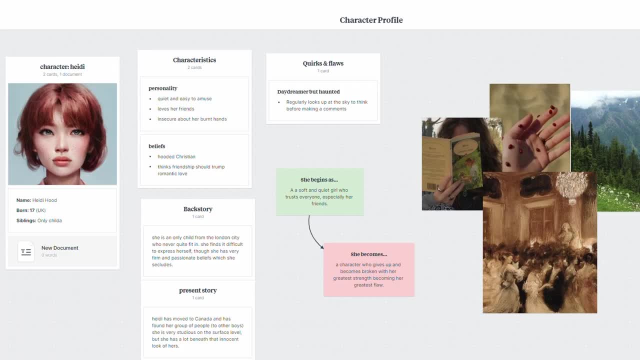 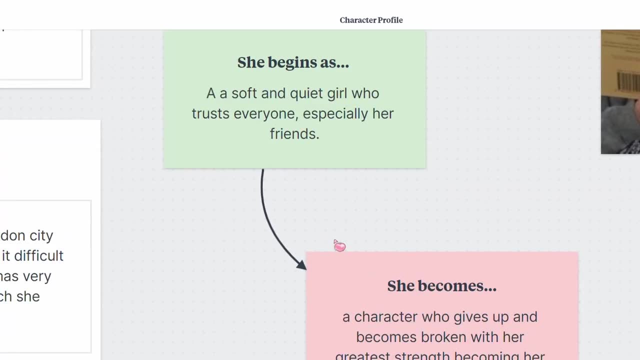 here we have heidi. i adore her. this, literally, is like my favorite page ever because i love characters. if you guys have watched all my videos, i love characters. i love especially this little part which shows like a sort of direct- um yeah, sort of link between what your character is and how your character has been throughout the book, and also 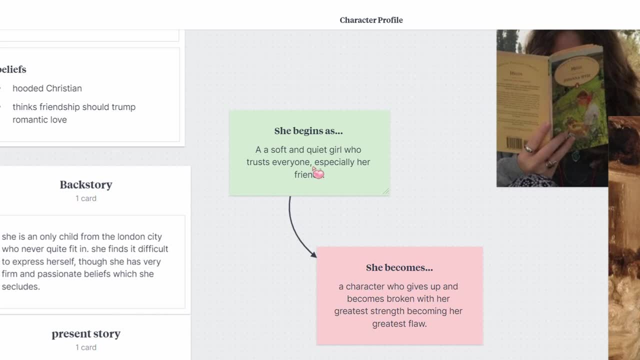 what is your character and how it's related to me personally. so i know a lot of people like to have a positive reaction to that and i love this part of the book. i really do love this character and by the time i get to the end i actually want to share the clinical story along with it. 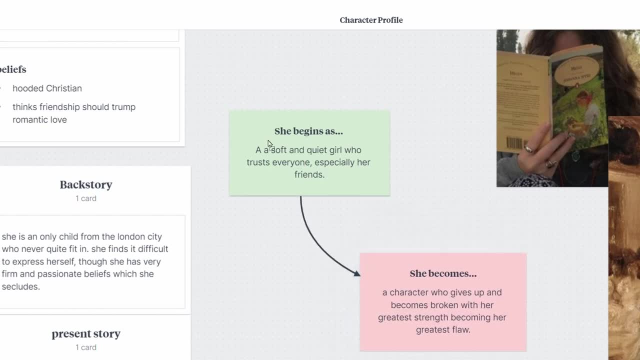 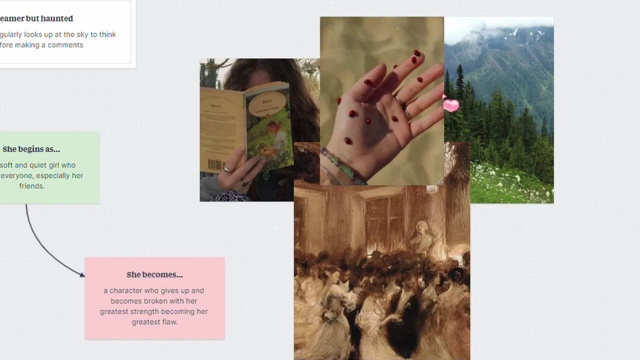 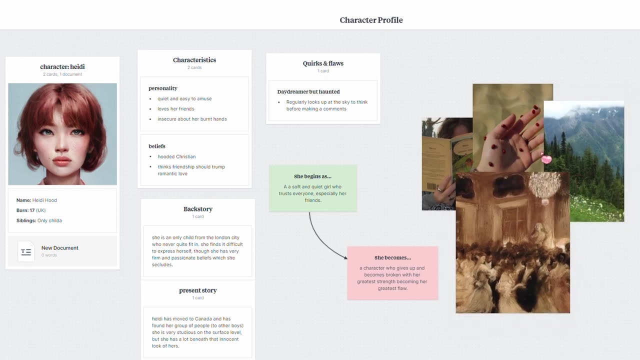 what they become so like. this sort of interactive stuff is so fun to me and the fact that you can create little vision boards like this and you can just move everything around so easily. it's literally just such a interactive space and a very creative space for writers like us. but anyways, i'm 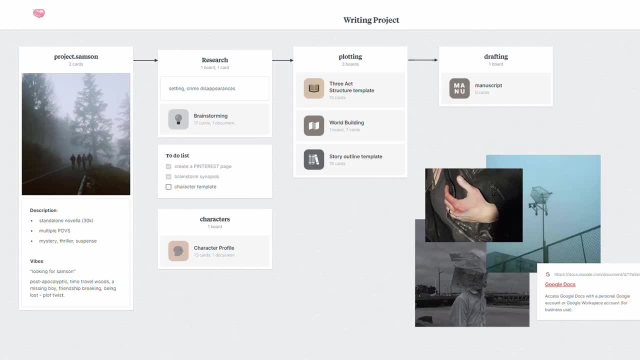 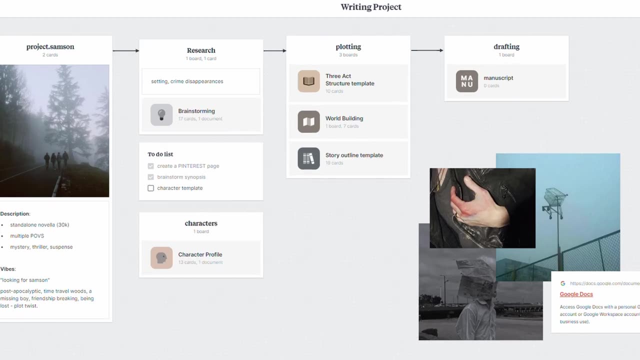 gonna go to my um home page and this is what it looks like. again, you can just create these boards and it's kind of like a little bit of a home page, a little bit of like a website for your book, which is so fun. but anyways, this is me just giving a little bit of a tour and, yeah, let's go ahead and 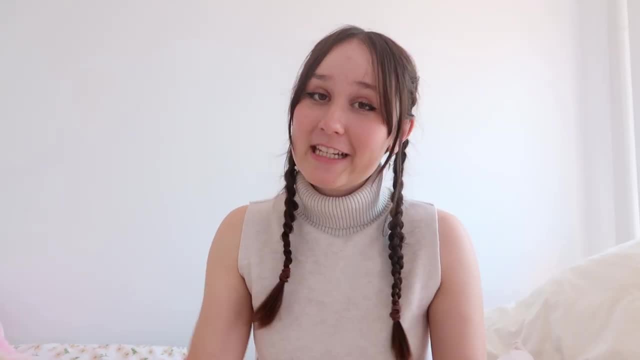 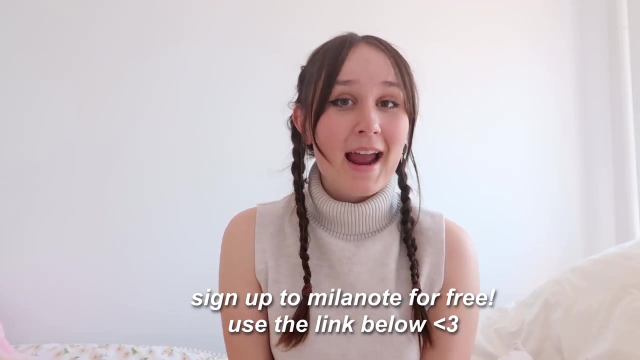 get on to the video. so Milanote, of course, is for free. if you guys want to check them out, definitely do down below and sign up to Milanote today. so, yeah, i really encourage you guys to check out Milanote and, yeah, thank you so much, Milanote, for sponsoring this video and making this video. 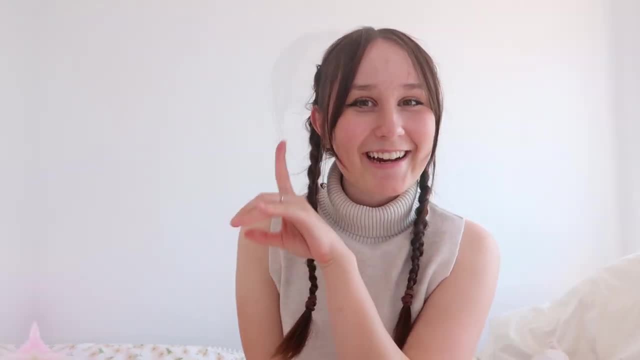 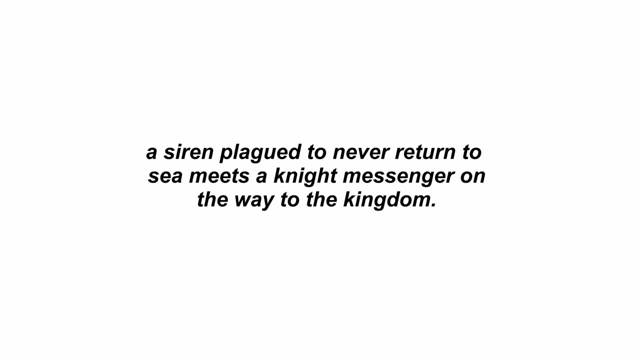 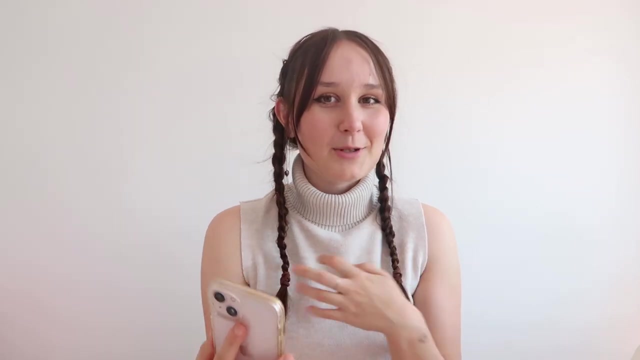 possible. let's go ahead and get on to the video. let's go. okay. number one: a siren plagued to never return to sea meets a knight messenger on the way to the kingdom. so, like, this gives me a little like a mythical vibes and it's like, of course, like a love romance between a knight and like. 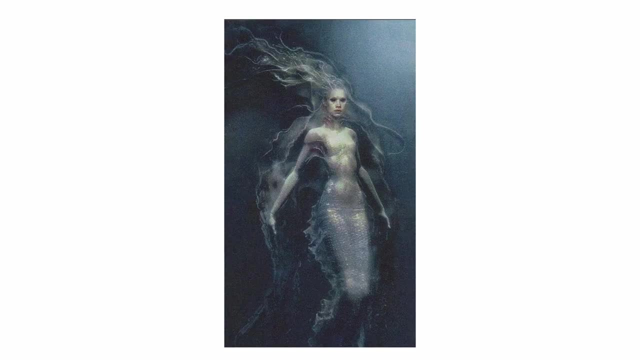 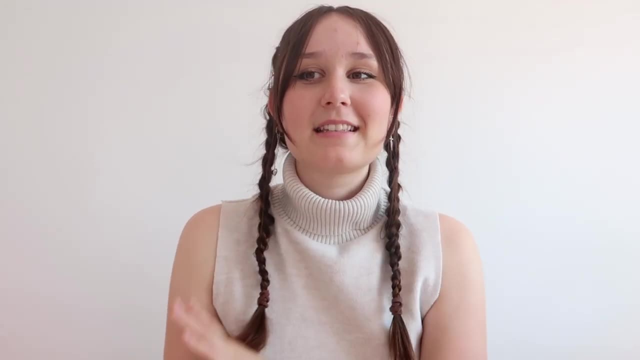 an upholder of the law and the mysterious siren. if you guys don't know what sirens are, they're kind of like sea creatures and anyways, yeah, she's kind of plagued never to return to sea. so she's kind of like a human disguised as a siren and i guess maybe in that world. 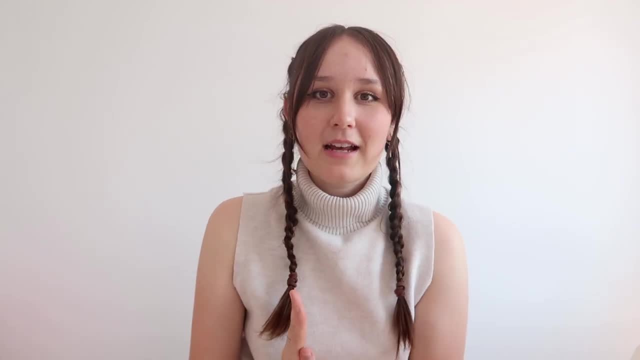 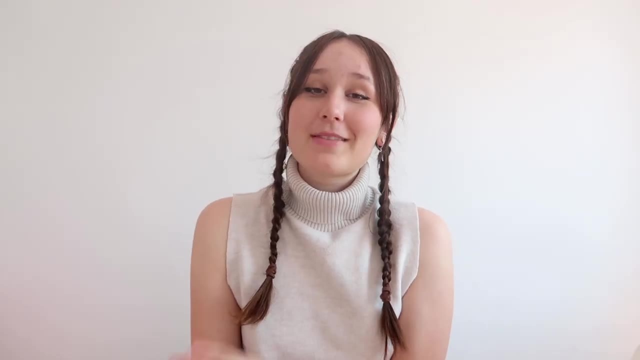 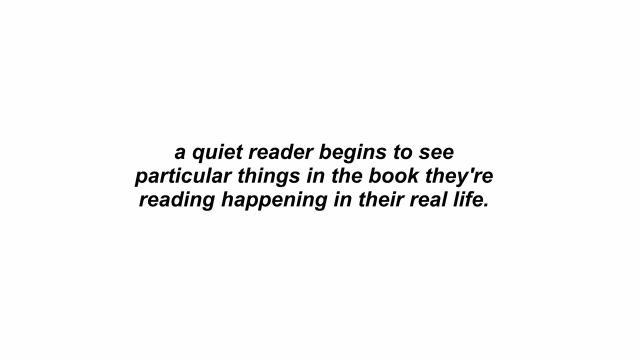 sirens are like witches and they can't be trusted and stuff like that. but the knight doesn't know. the knows that she's in trouble and needs to take her back to the kingdom. so that's really interesting. the second book idea is: a quiet reader begins to see particular things in the book they're reading. 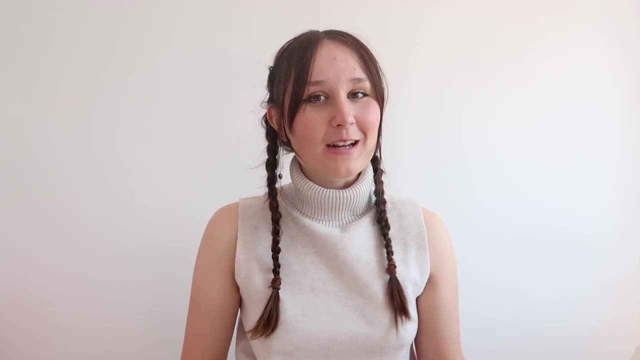 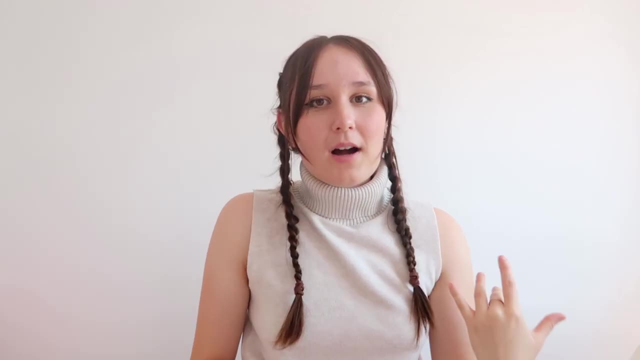 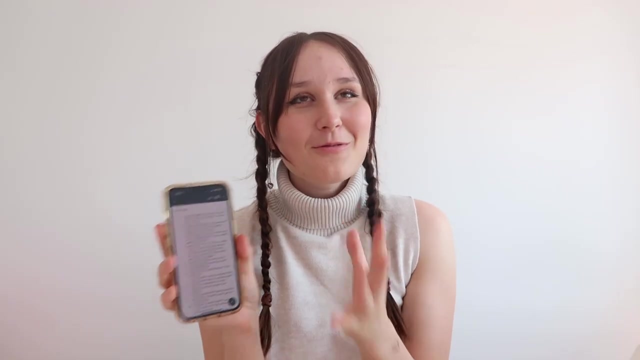 happening in their real life. this was my dream when i was like a 16 year old book nerd. um, i would just be reading my hurt books and just like, wow, like why can't i see this man in front of me? why can't he ask me to go on this adventure with him? but, like this sort of thing really does, i 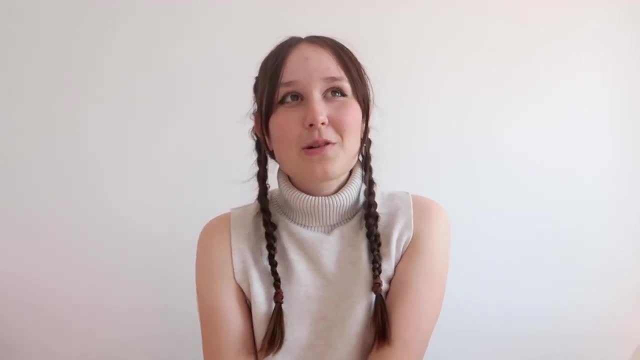 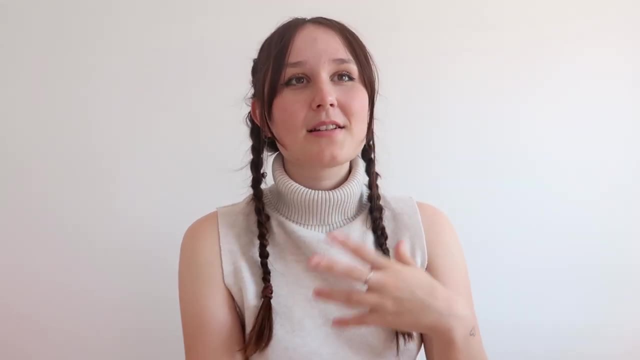 don't know, make me excited and something that's really like a fun, passionate project that i'd love to get into. but you can either kind of create new characters or characters of your actual books or maybe characters from other books, um, such as like the, such as like cassandra claire's, like shadow. 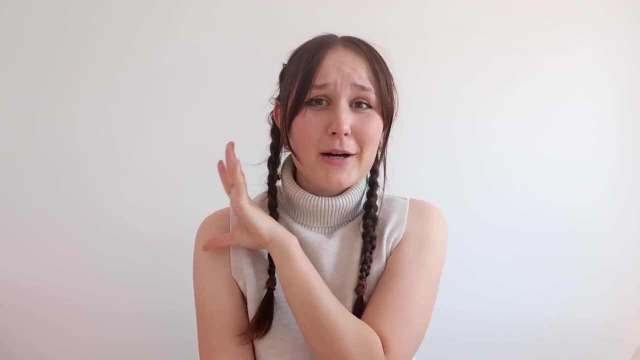 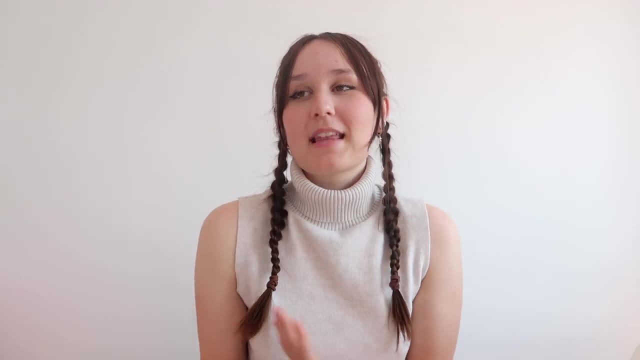 hunter world, maybe mixed with like the six of crows, labor dugo world, like those sorts of like characters and those sorts of plots like thick and mean in this real person's world. like that would be so cool. the third book idea is: a young mage is. 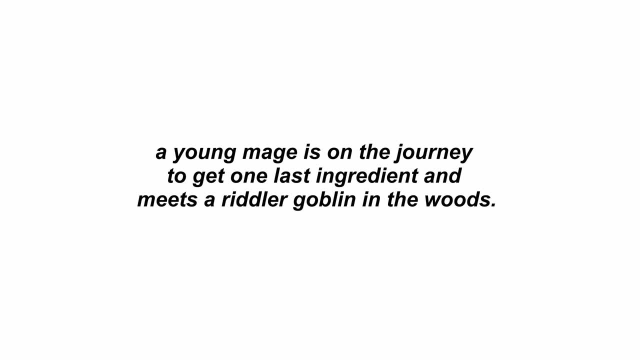 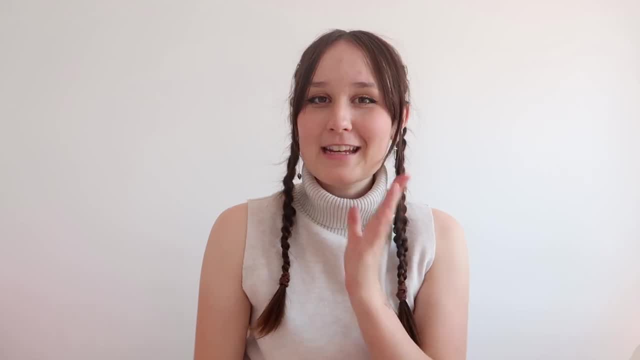 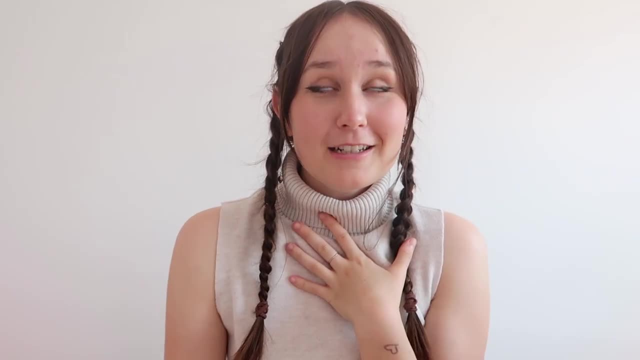 on the journey to get one last ingredient and it meets a riddler goblin in the woods. this seems like more of a short novella sort of a mysterious sort of book that seems so fun to write, especially with the riddle part and a riddle gobbler, gobbler, riddle gobbler, a riddle goblin, um, and it gives me 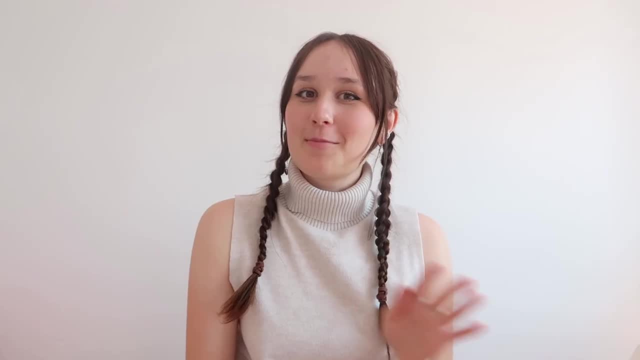 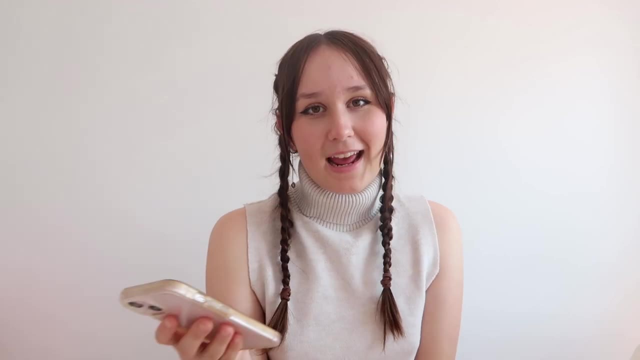 vibes of smeagol and the lord of the rings and the lord of the rings and the lord of the rings, and i am all here for it. i think it'll just be such a fun little thing. um, and yeah, number four, a white haired boy, because i love white head boys. so a white haired boy who is a trainer in a fable. 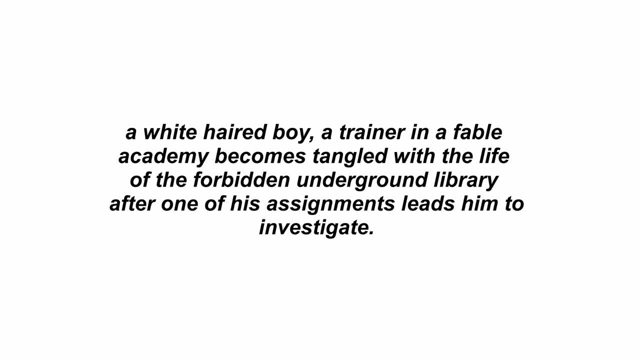 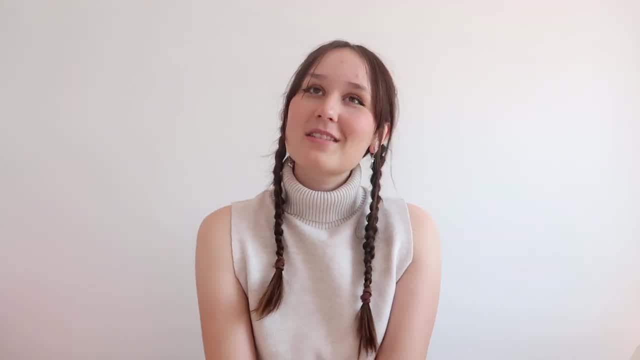 academy becomes entangled with the life of a forbidden underground library after one of his assignments leads him to investigate. so i think this would be really interesting. lots of like magic, lots of like laszlo, strange vibes, um, you know, that's sort of like aesthetic or 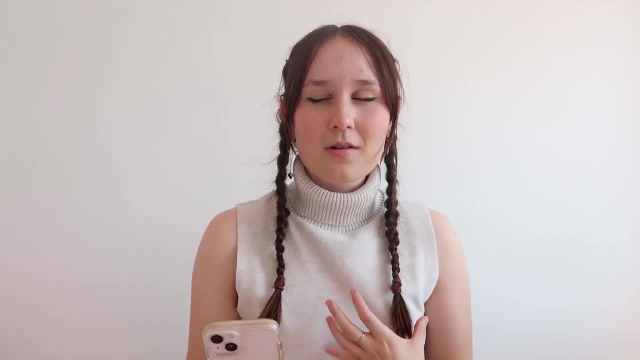 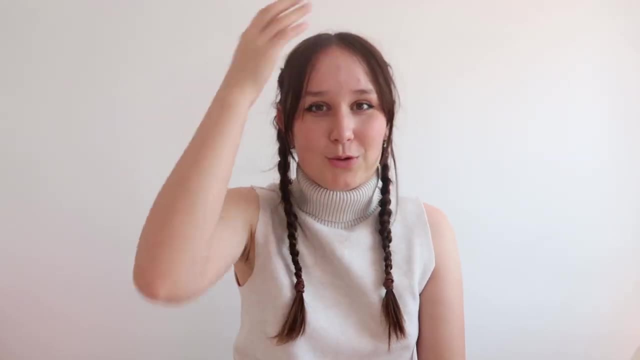 policy, like those sorts of vibes are very, very cool and i think, of course, forgotten underground library, yes, and especially like it's tied into his assignment and how like maybe that will lead to something mysterious or something like that. i think that'll be so fun to just explore. 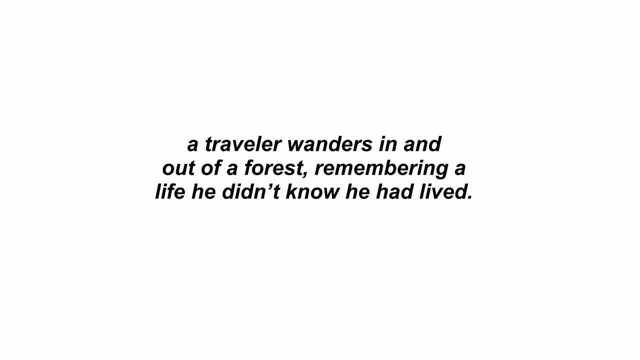 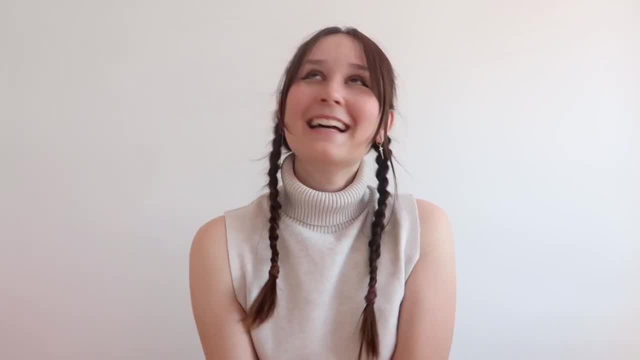 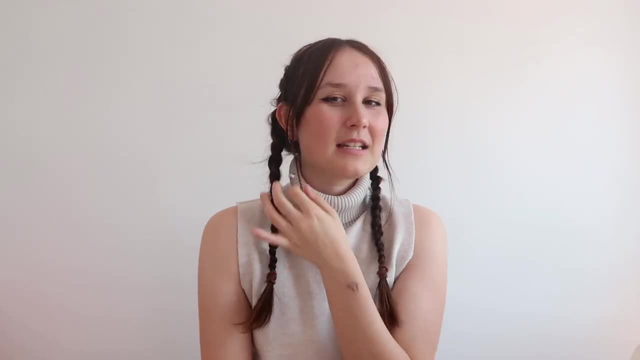 number five: a traveler wanders in and out of a forest remembering a life he didn't know he'd lived. okay, why did that slay? that sounds so fun, like how mysterious and how like how much fun you can have with like the creativity in this book and how like different. 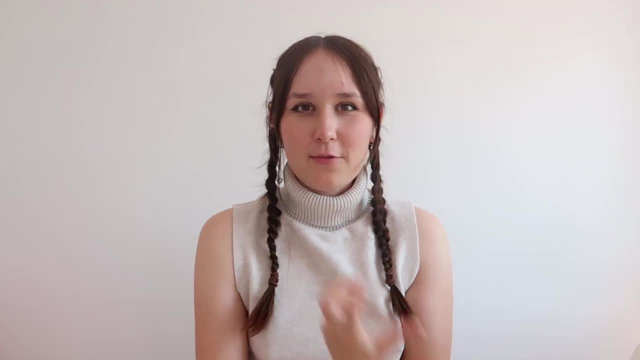 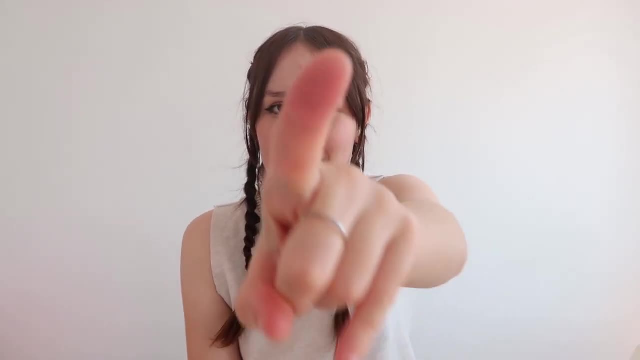 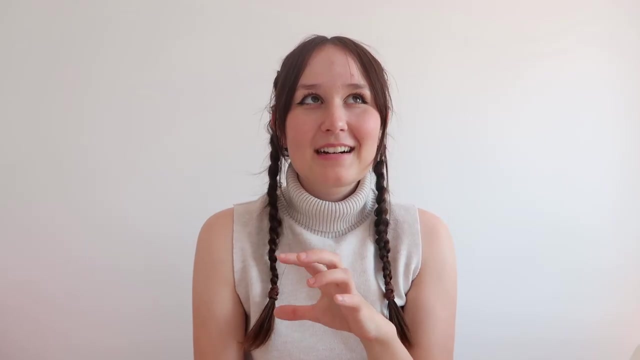 lives, yeah, and like how this wonderer, like what was his life before he started wandering. oh my gosh guys, i also just watched a movie- it's like a polish movie on netflix. go watch it. it made me cry. um, it's called a forgotten love and it's the most wholesome thing where like the main character. 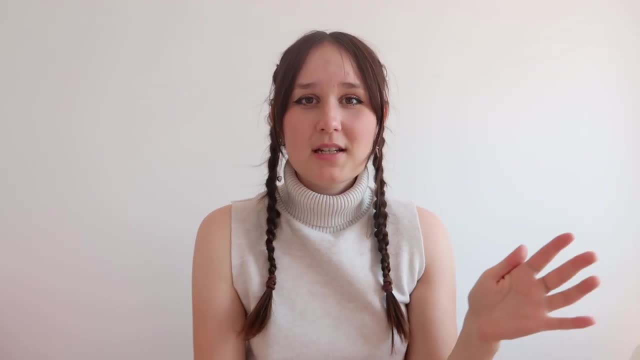 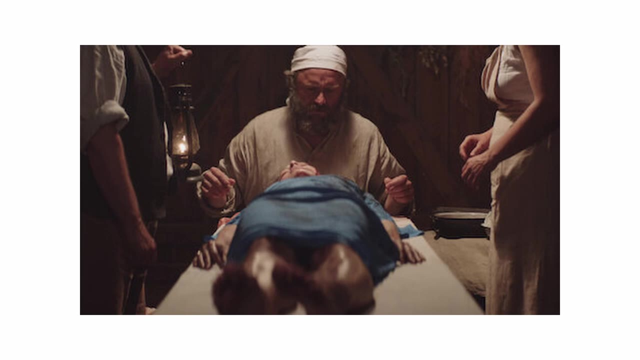 is a doctor and he gets beat up and like: has amnesia, so he like wonders and doesn't know what he's looking for. but then he ends up like remembering his life and he's like: oh my gosh, what's up, what's going on. and he's like: oh yeah, i'm a doctor and i'm a doctor and i have this. 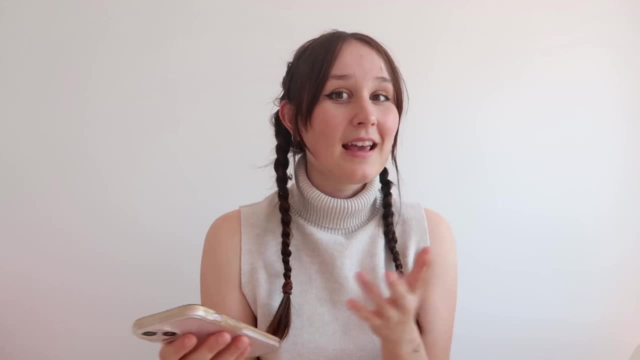 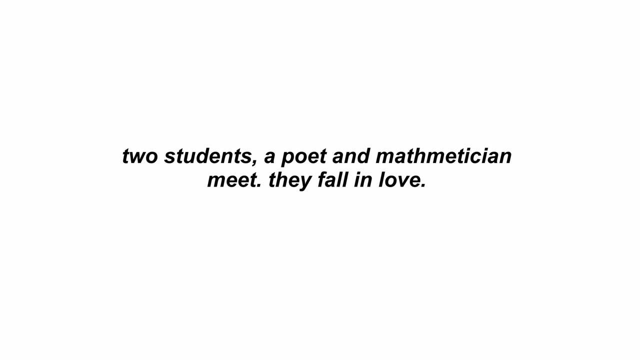 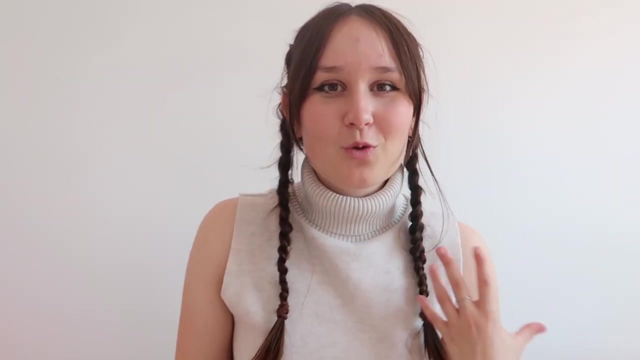 sort of skills, of being, you know, a sort of doctor. so it's kind of like interesting, like his half life and maybe, like this person has amnesia and they start to remember things, number six: two students, a poet and a mathematician, meet and they fall in love, of course. i think this is just 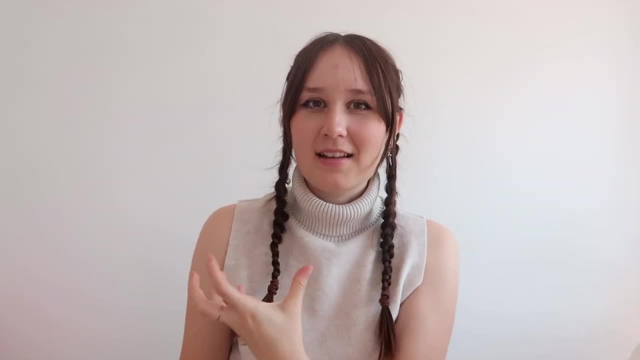 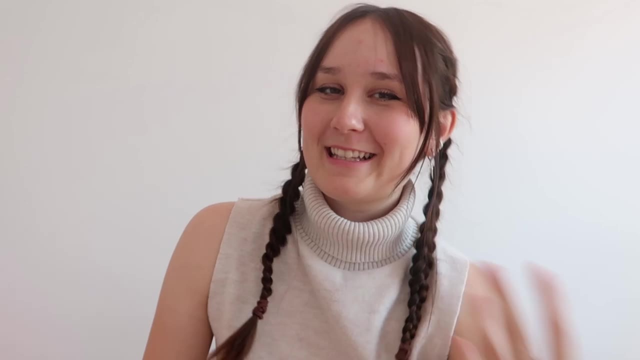 so fun and just seeing, like the i don't know potential romance and the different ideas of like how the characters are, like like a poet and how like pretty his. i don't know the way that they speak and the way that they view the world is so different from. 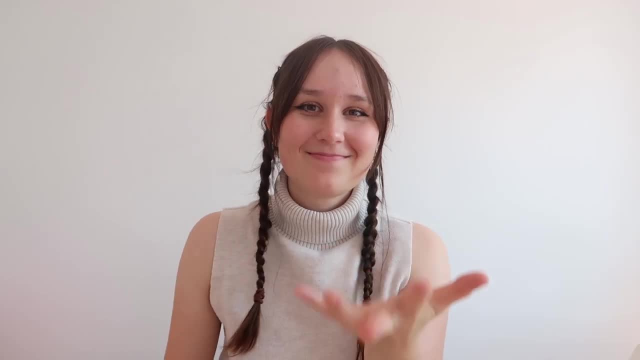 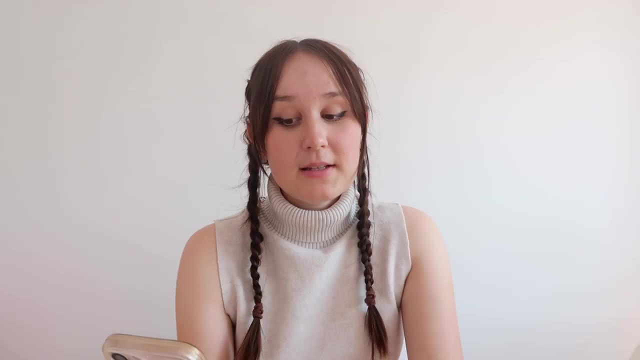 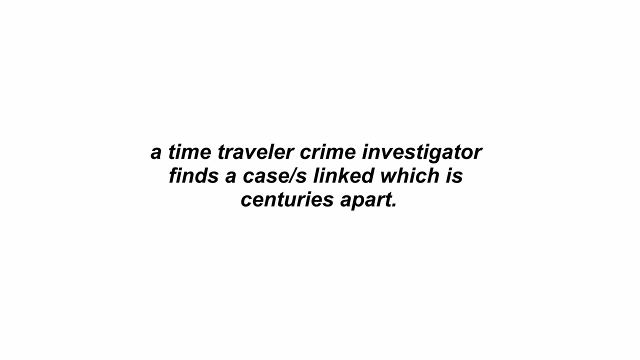 the mathematician who's so like straightforward and so like: take, take it please. please write it so i can read that romance number seven: a time traveler crime investigator- that seems cool- finds a couple cases which is linked from centuries apart. this sounds really fun. i remember brainstorming it. 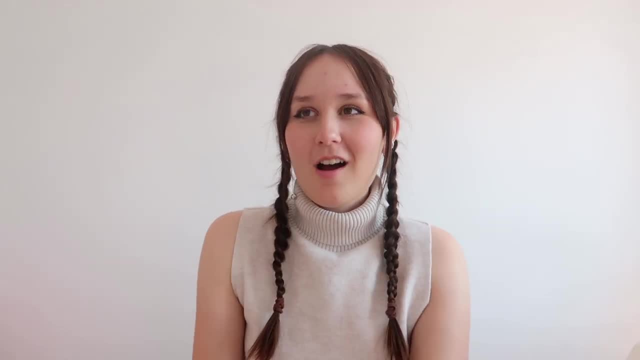 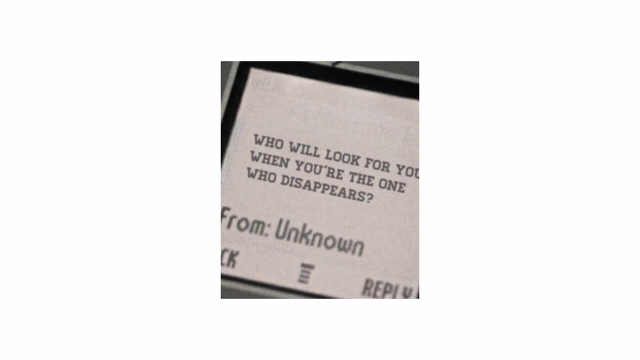 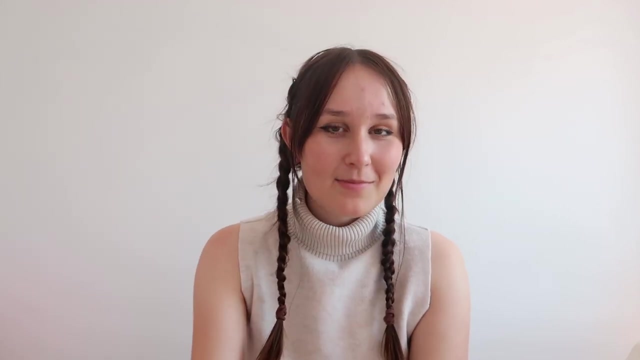 with someone and just kind of like thinking about the potential of like this cool like agency where they time travel and try to solve mysteries and solve, uh, crimes and different cases from like centuries apart, maybe like one like involves them somehow causing the crime in some sort of other. 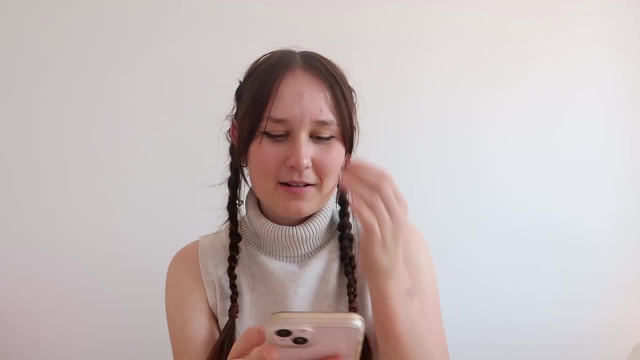 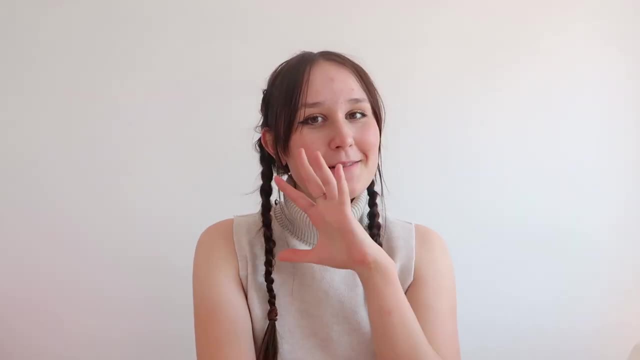 time. like: isn't that epic? isn't that epic? number eight: a grave is unearthed at a magic academy, just as a student goes missing. this gives me look lee wright. vibes, like if you guys know lee wright's on instagram. like this gives me vibes, i think, maybe. 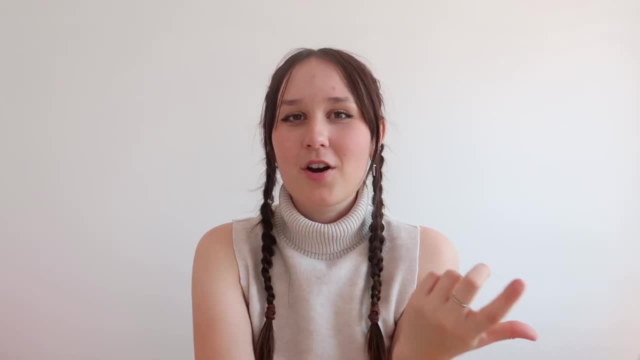 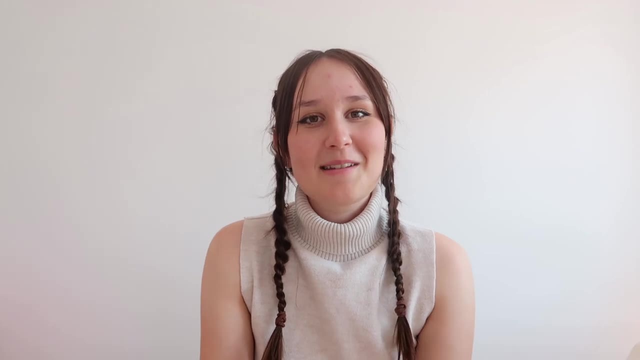 her story is kind of similar to this but like i know there's like a grave getting unearthed, um, but this seems mysterious. like i love sort of duck, duck, duck, academia, duck, oh number nine. okay, it's an alice in wonderland retelling, where the characters 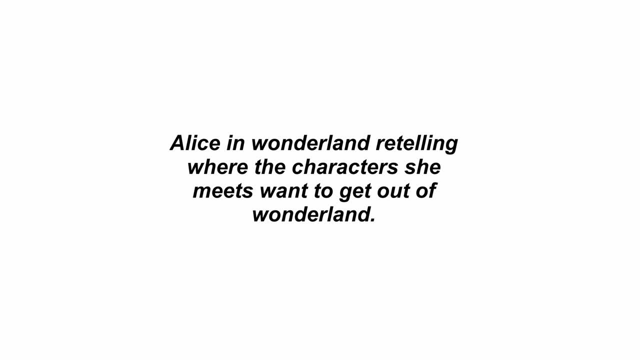 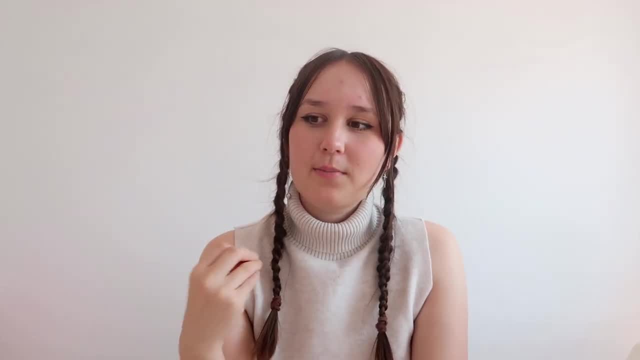 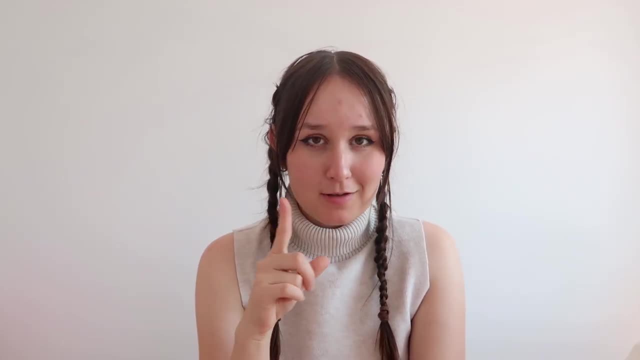 that alice meet actually want to get out of wonderland. isn't that interesting? because like they kind of like want her to stay kind of and slay the beast, but maybe they want her to like be her savior, but in another way sounds really cool. okay, let's move on to the next one, number 10: a celestial powered object. 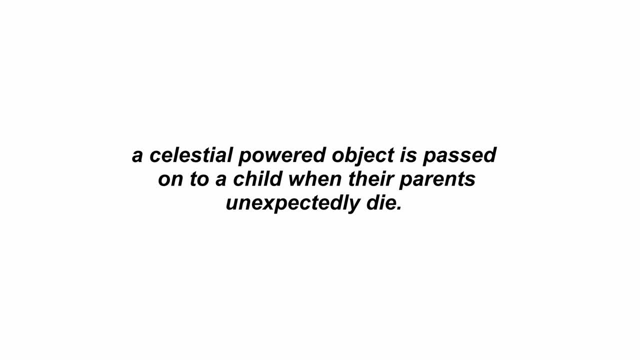 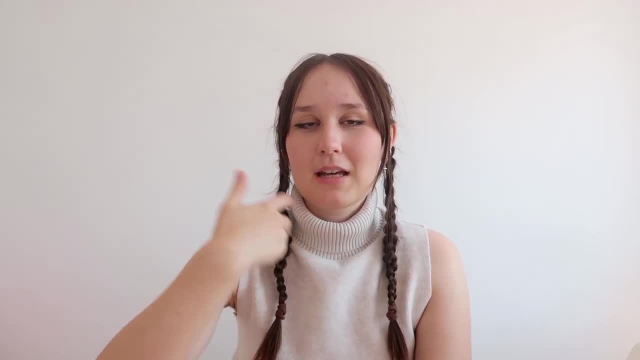 is passed onto a child when their parents unexpectedly die, and i think this gives me vibes of like harry potter, where you know, harry potter, he doesn't really know that he's, uh, a model. no, he's a wizard. you're a wizard, harry, of course, um. 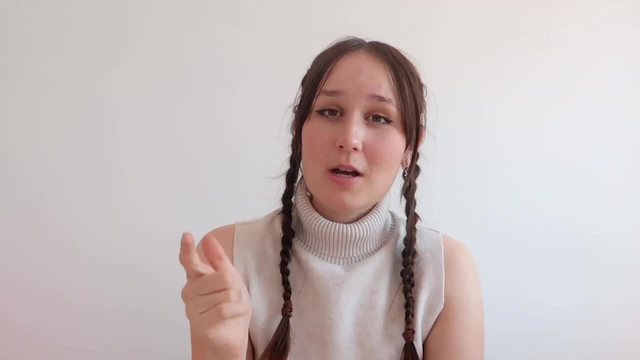 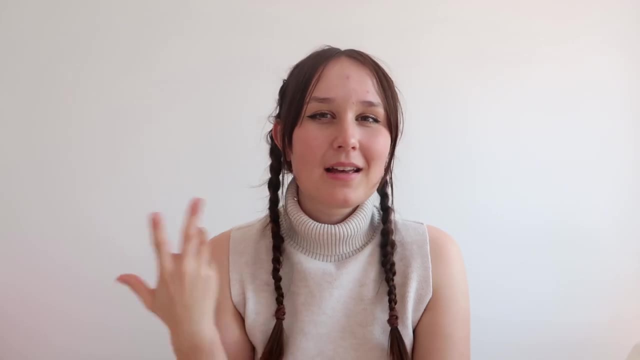 and like this sort of vibe, like it kind of is really similar to project gem spell, which is one of my books that i have neglected to write um, but it gives me that sort of aesthetic where it's like these interesting powers like i have, there's a whole world that i don't know. wow, why did my? 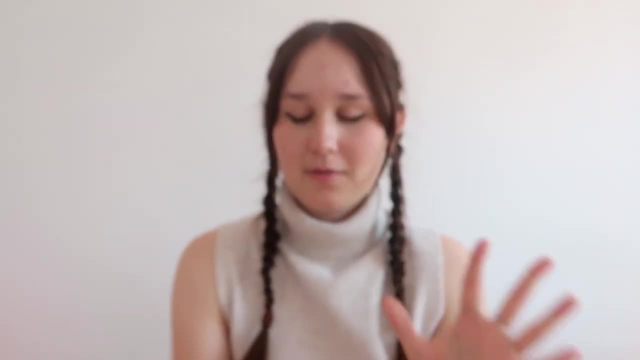 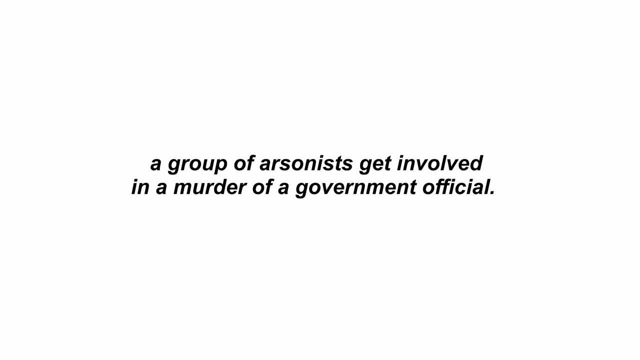 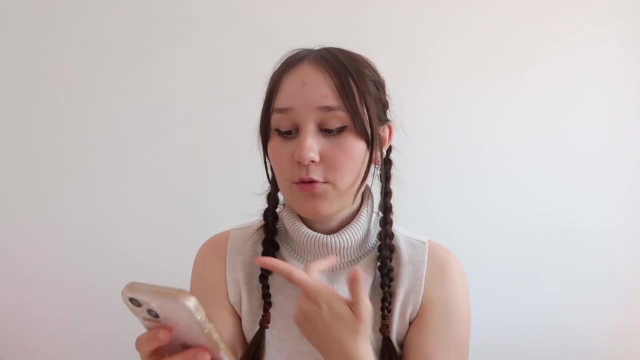 parents tell me i resent them but kind of want to know more that sort of aesthetic, you guys. you guys know what i mean. okay, let's go. um, oh, oh, this is fun. a group of arsonists get involved in a murder of a government official. i i'm gonna write that today, like that sounds so cool and like the. 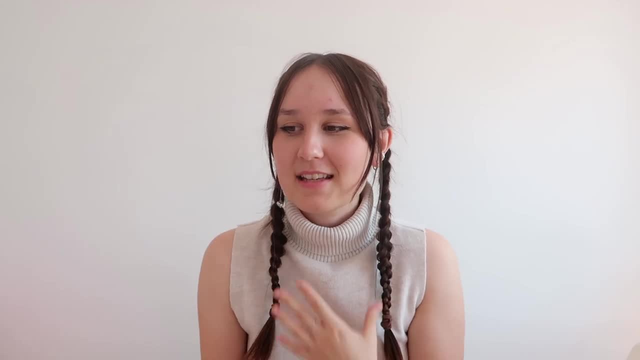 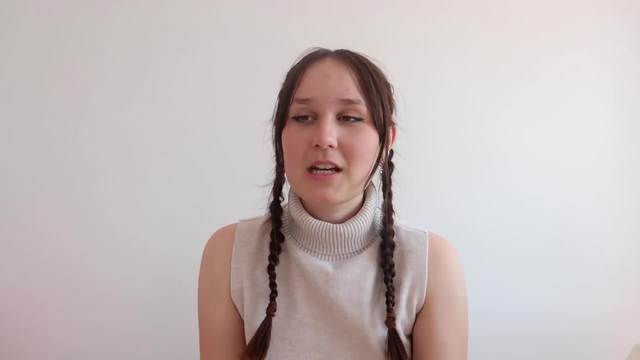 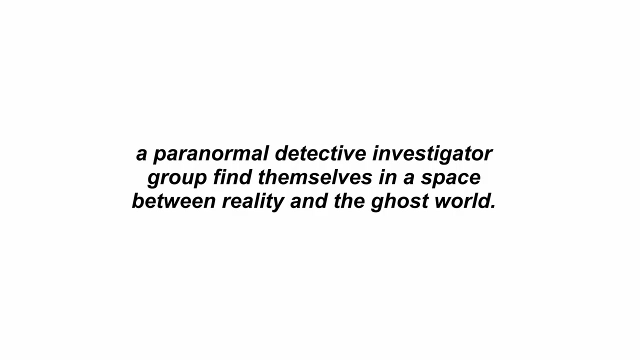 politic, like the politics intrigue and like arsonist and how like that's linked with like crime and like the murder, oh and like, maybe like family sort of connections. these are some good ideas, okay. number uh 12. number 12: a paranormal detective investigator group find themselves in. 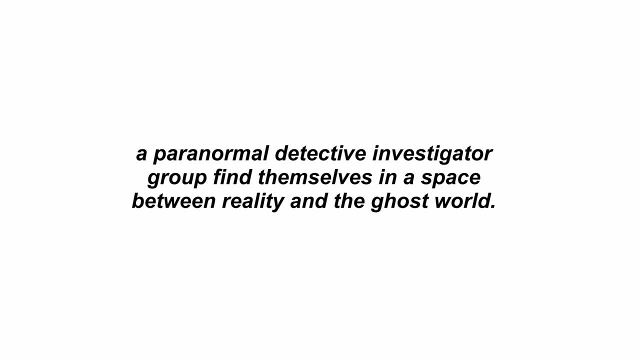 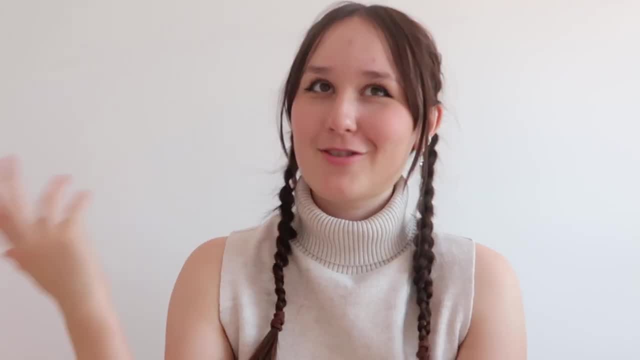 a space between reality and the ghost world. wow, that sounds fun. like can you imagine? like gives me like stranger things vibes again. like this will just like gives me vibes of like all these different shows and like books i've already read and watched. so that sounds fun and like i love ghostbusters. 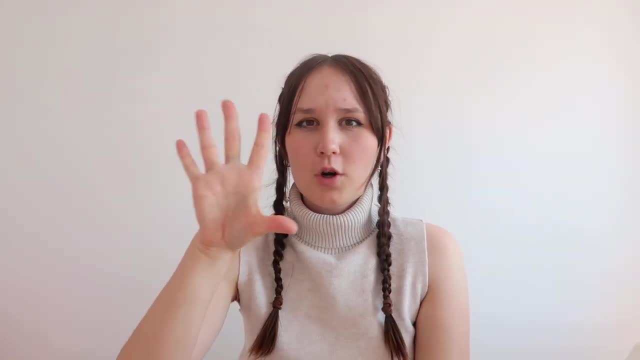 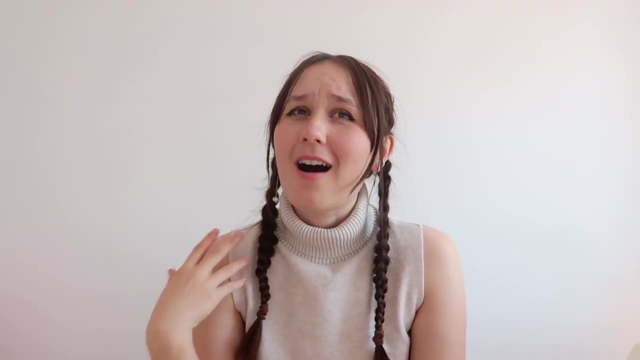 oh wait, what's that? oh sorry, my brain. lockwood and co. that is such a good. i really want to rewatch it. i hope they come with a second season, but i don't think they are. it's a netflix series. there's some really good netflix series, but lockwood and co- that. 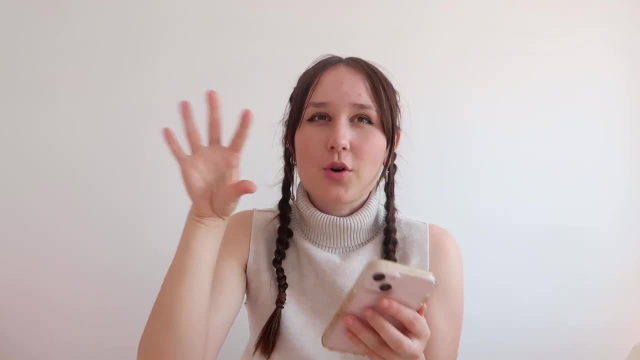 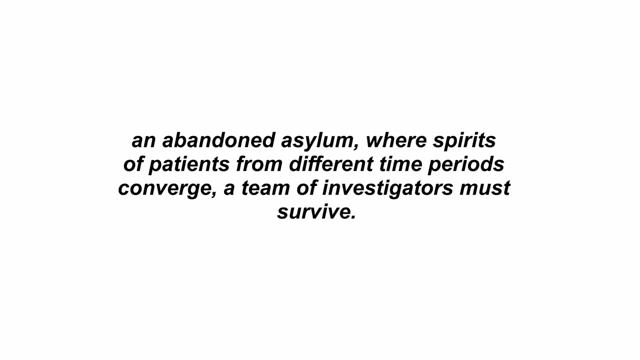 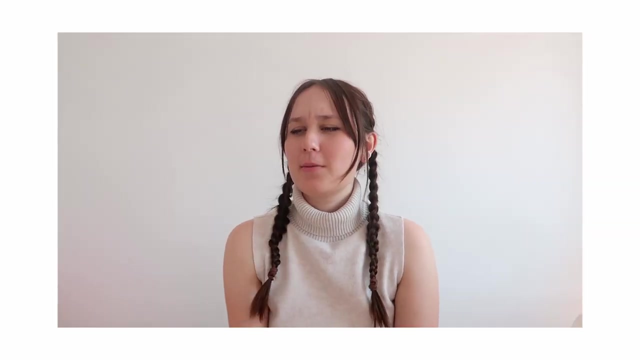 gives me that vibe. so good, so good. they're like ghost hunters who can like see ghosts. so cool, so freaking, cool. number 13: we have an abandoned asylum where spirits of patients from different time periods converge and the team of investigators must survive. that's so cool. like dead people- wait, not dead people. are they dead? 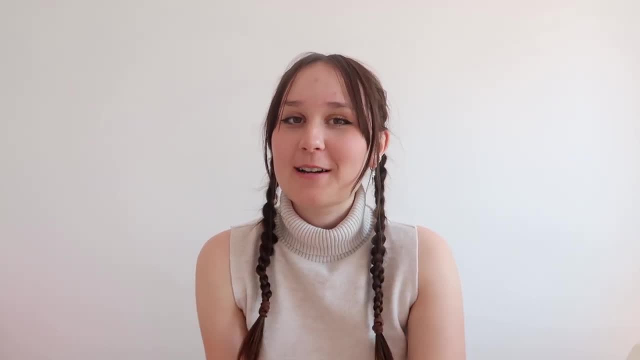 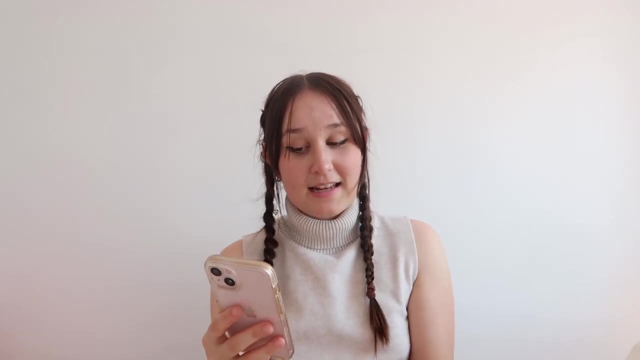 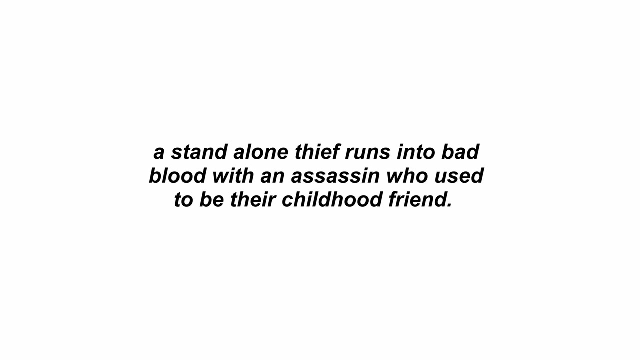 but spirits of patients from different time periods converge. that's so cool but kind of scary, like i would probably be scared reading that book. okay, number 14: we have a standalone thief who runs into bad blood with an assassin who used to be their childhood friend. i think like a like a love romance can bloom in here. i feel like it would be. 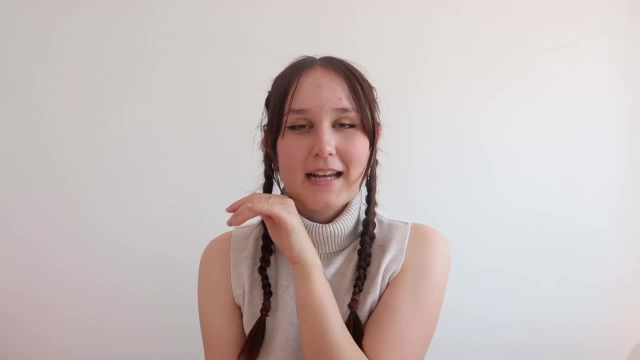 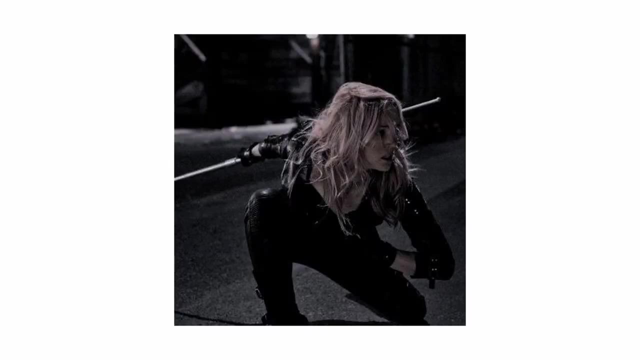 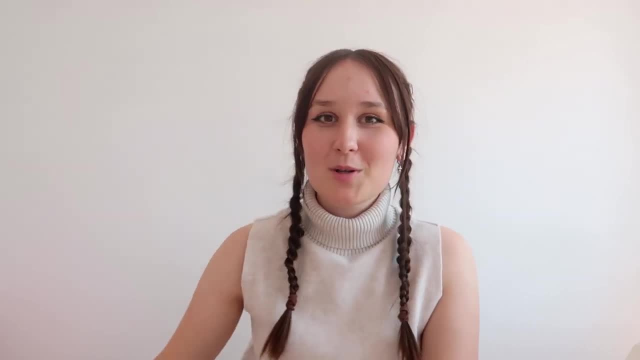 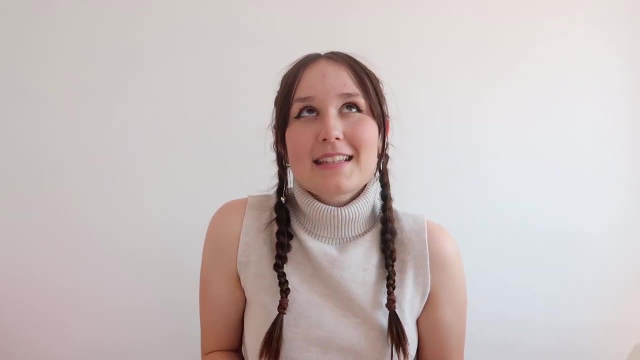 know when they might end up work together, but i don't know a bunch of time period. an assassin and they promise to like serve the world, but one of them turn into assassin. one of them turn into a like a thief and they kind of had bad blood but then kind of like maybe you have to work together. 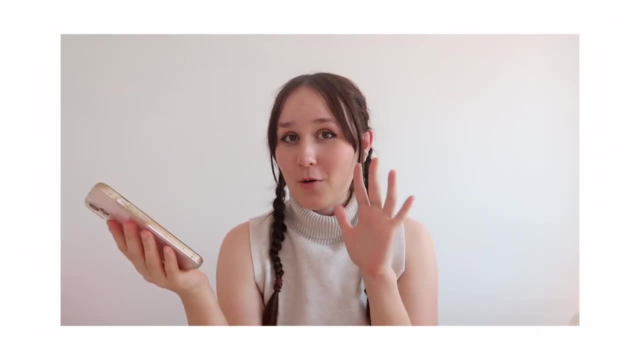 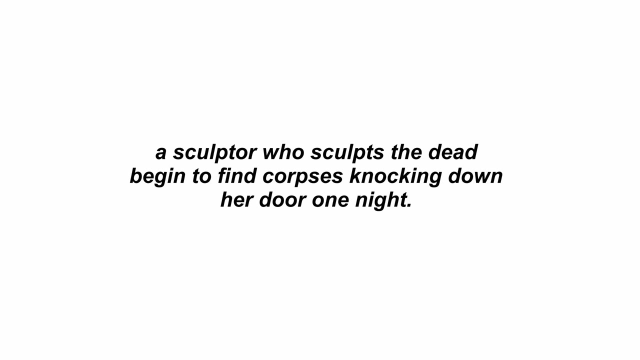 that sounds so cool. an assassin working with a thief- again, i don't approve of stealing or killing people, but that's epic, okay. next we have number 15, which is a sculptor who sculpts the dead begin to find corpses, knocking down her door one night. 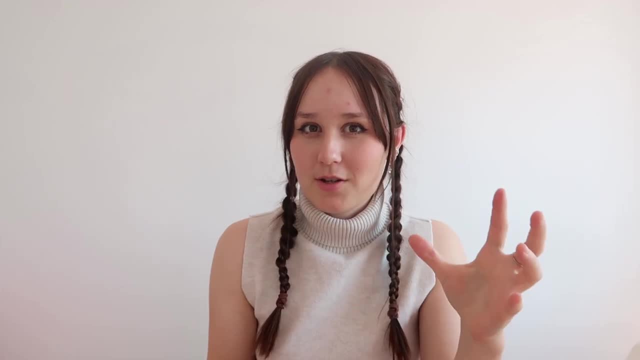 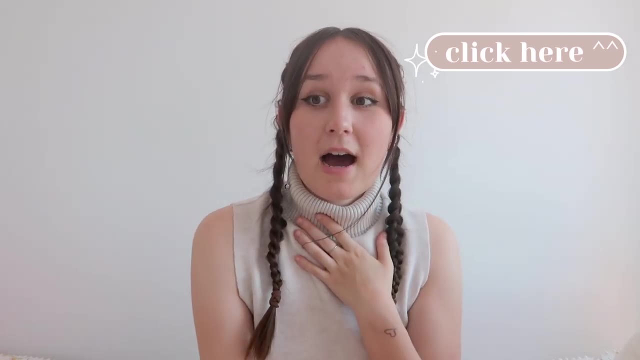 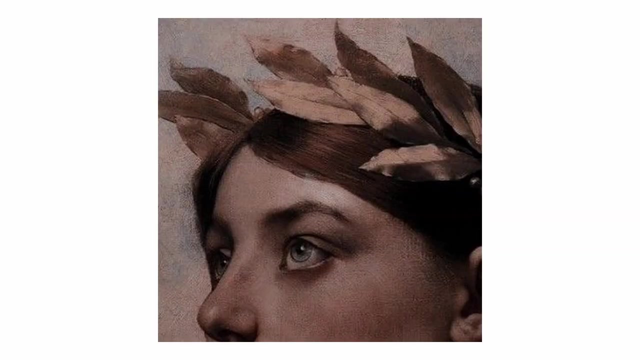 rest my case. i love the sculptor aesthetic. i love it so much and actually i think i do have a podcast. if i can find it i'll link in the description or the icard where i actually have a really cool short story where it has it follows like a sculptor who basically sculpts this like the god of nike. 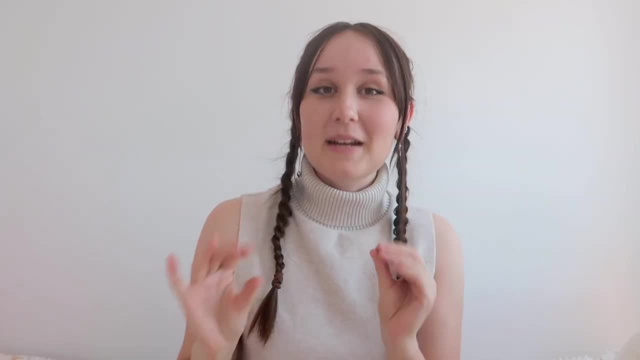 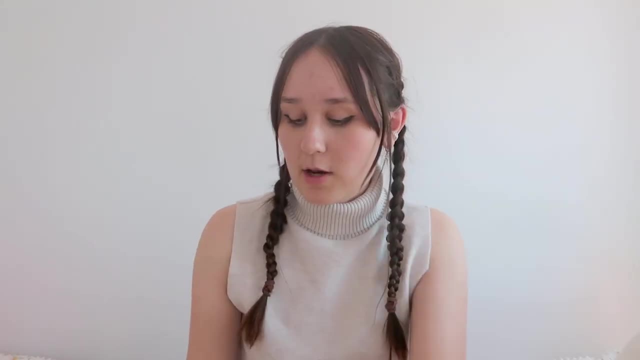 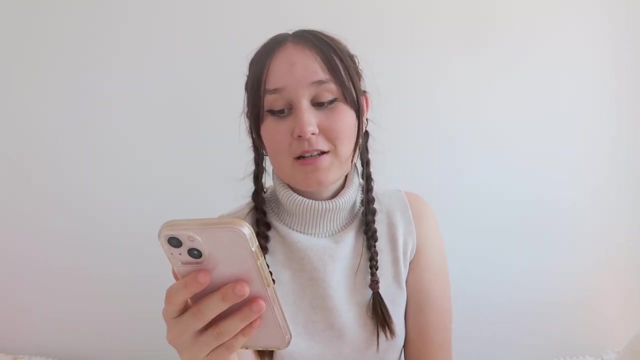 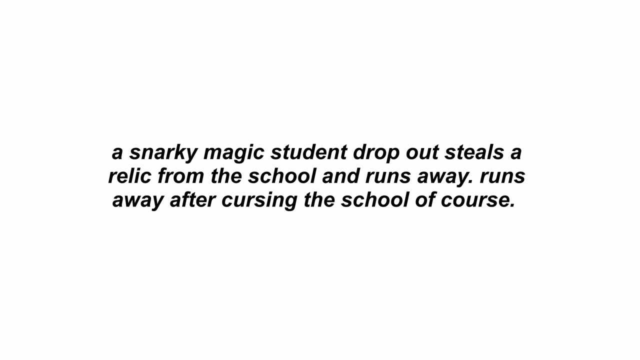 what is my voice? basically, she sculpts the god of nike and then she goes to the museum to see like that statue. anyways, go check that out. anyways, let's continue. number 16: we have a snarky magical student dropout, steals a relic from the school and runs away. runs away, of course, after cursing. 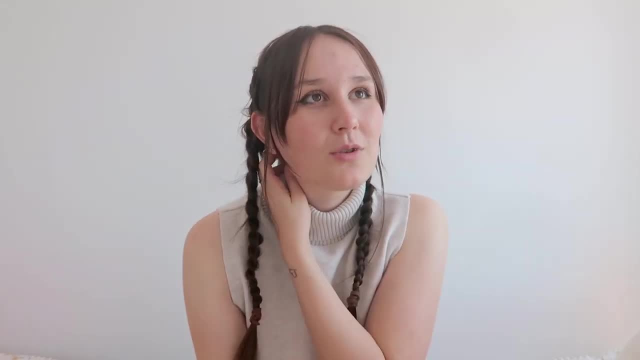 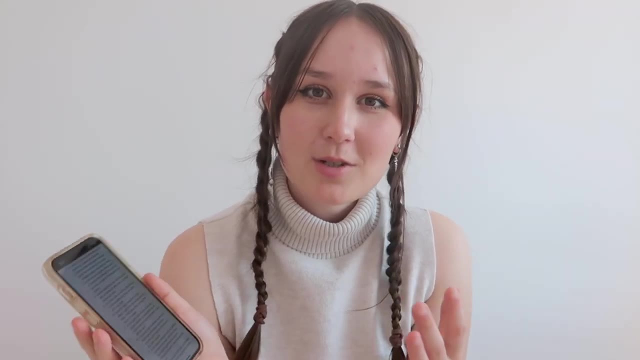 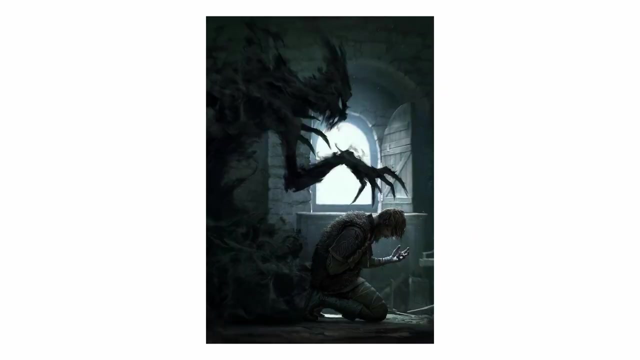 the whole school. this is actually a story i wanted to start, so a lot of these ideas are actually books that i have started, but not um committed to. and it's called like asara keys, who's like the main character and and she basically curses the whole school, i think, and basically like no one remembers her but one. 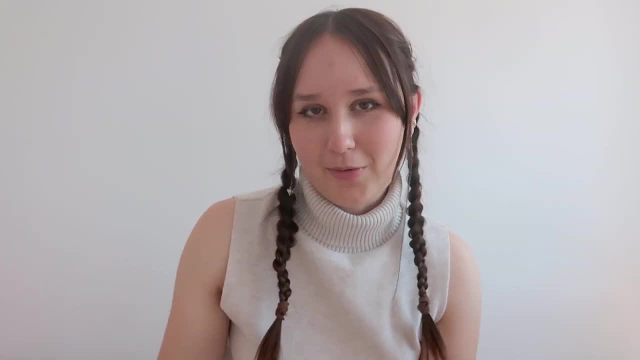 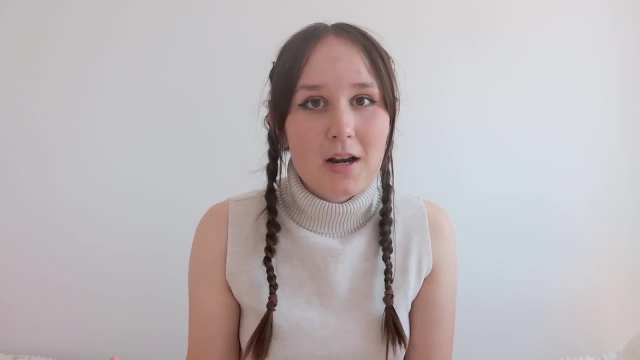 boy for some reason. i of course i don't know, because i didn't write the book and i it was just an idea and i was like writing the first chapter, and i think that's a tip also, if you guys get so excited about a new idea- which you probably are in this video- and if you do have 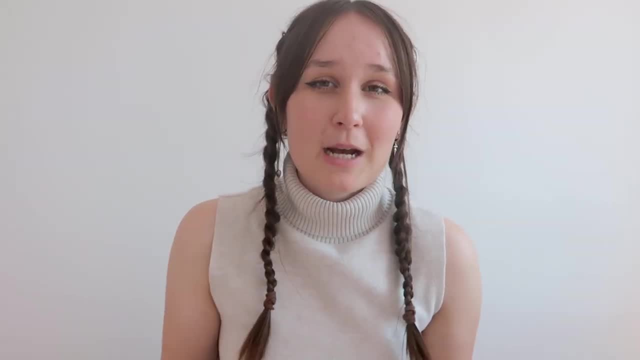 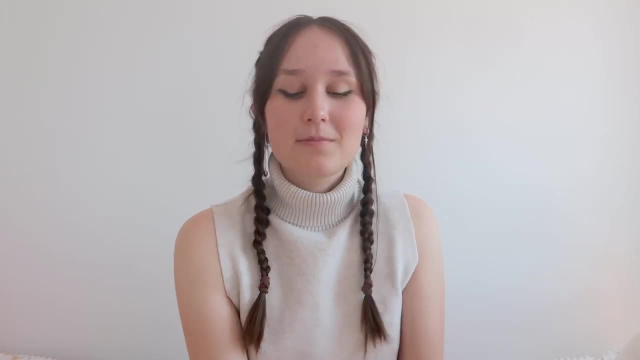 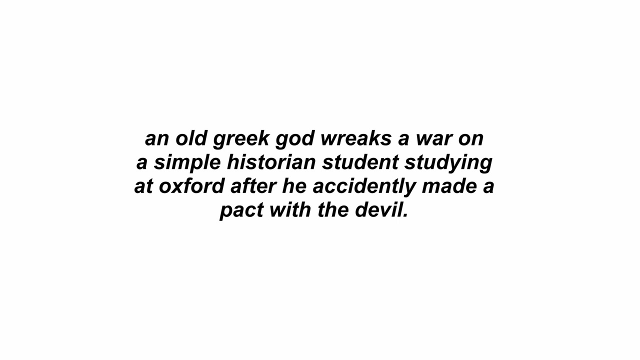 commitments. i encourage you just to write the first chapter, or first few chapters, if you really want to just get it out of your system. don't even plot it, just like write the first chapter because that just seems so fun. but anyways, that's the idea number 17. an old greek god wreaks a war on a simple 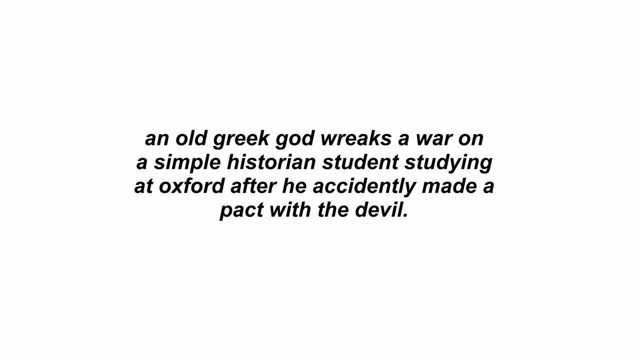 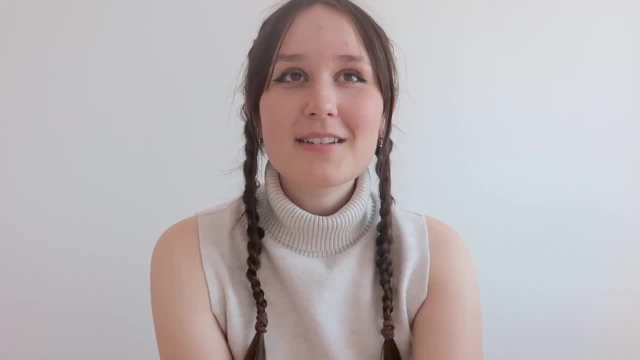 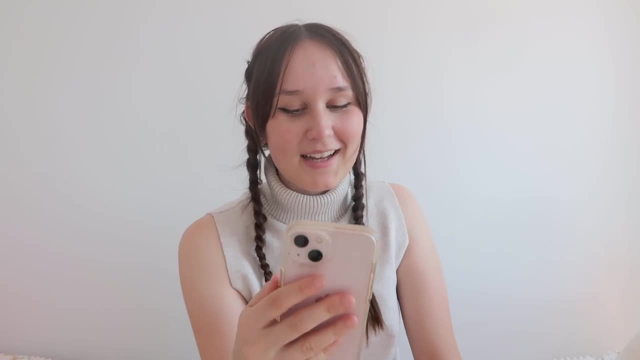 historian student studying at oxford after he accidentally made a pact with the devil- i'm not sure if it's a devil, maybe with hades- hey, hades, why does my voice crack? i'm not a teenage boy anyways. yeah, so that seems, seems really fun. like, doesn't that seem fun? that seems fun. um, okay, let's. 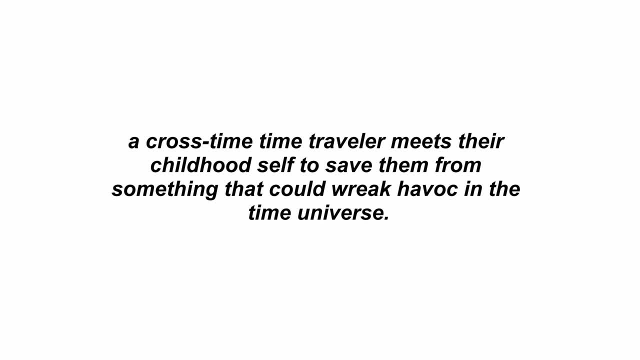 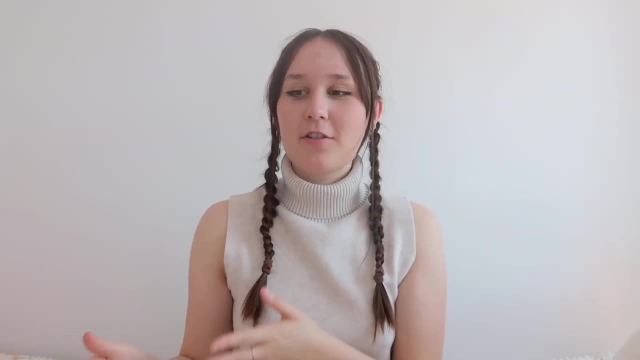 move on number 18. across time time traveler meets their childhood self to save them from something that could wreak havoc in the time universe. this gives me, like you know, time travelers like vibes. that seems so cool, though, like you're going back in time to like: save your childhood self, but you're able to like. 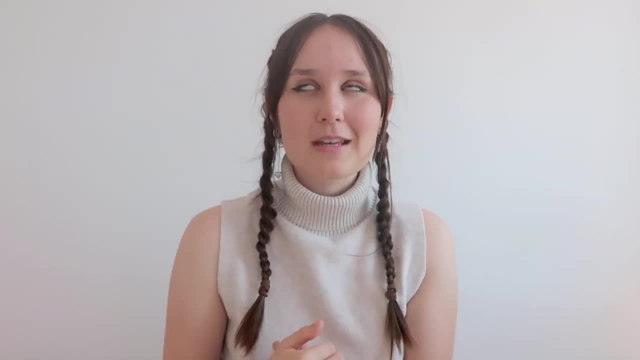 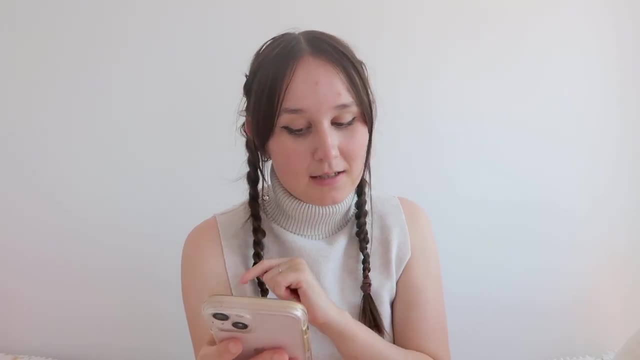 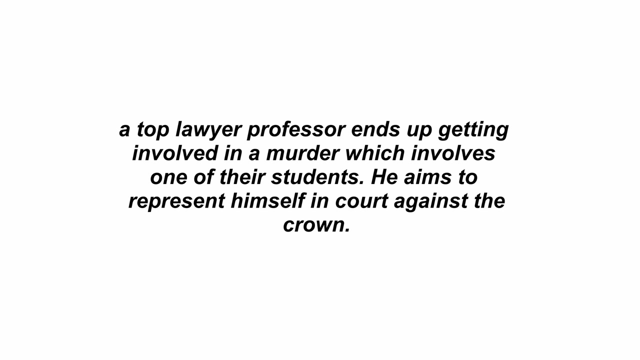 meet them in a way like it gives me like the terminator vibes in a way. um, that seems so cool. okay, we have the last two, which 19 is the top lawyer professor ends up getting involved in a murder of one of his students. he aims to represent himself in court against the crown, and i think this. 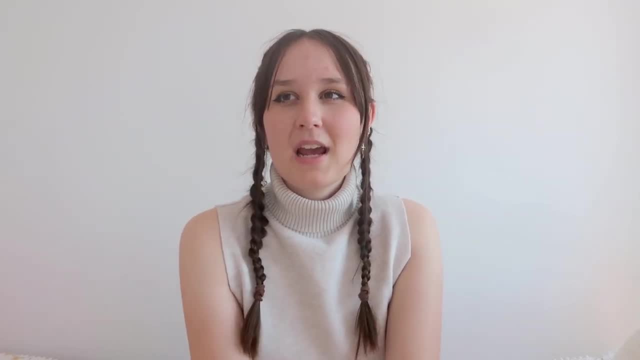 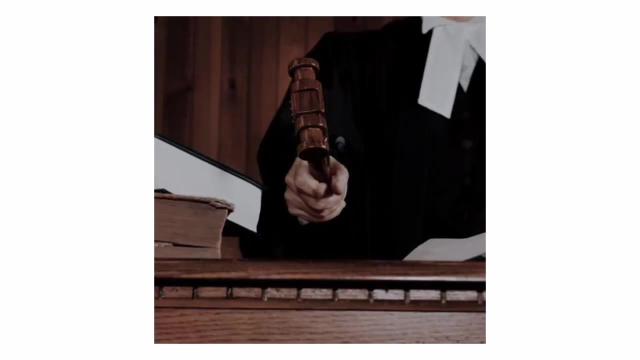 is really interesting. it's kind of like i don't know, touche, cliche, touche, what does touche actually mean? but basically, yeah, it's just kind of like interesting that it involves one of his students and maybe he's like a crime professor. i'm studying crime right now and i just actually got off a call. 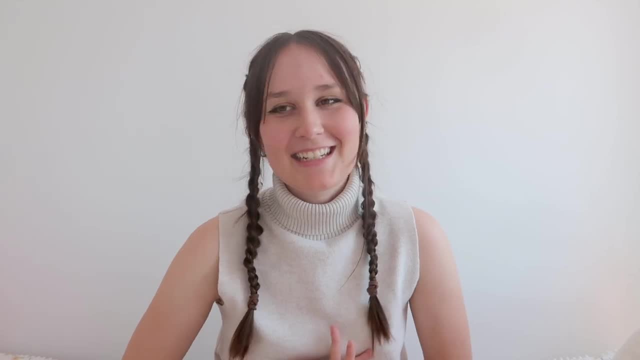 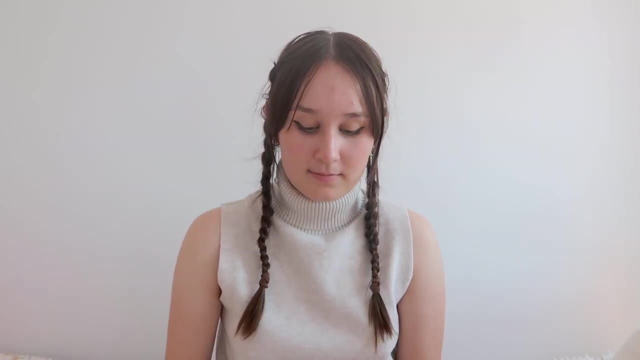 with one of my crime professors and like, very interesting, i did really bad in the exam and he was just telling me how much work i had to do to get to this point and i was like, oh my god, i'm i need to do for the next exam, but anyways, um, maybe i'll be them, i'm kidding, i'm kidding anyways. 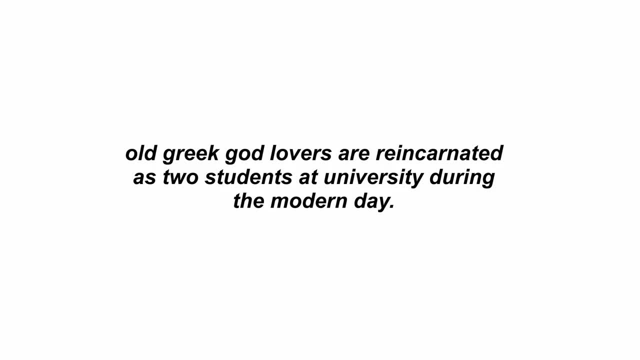 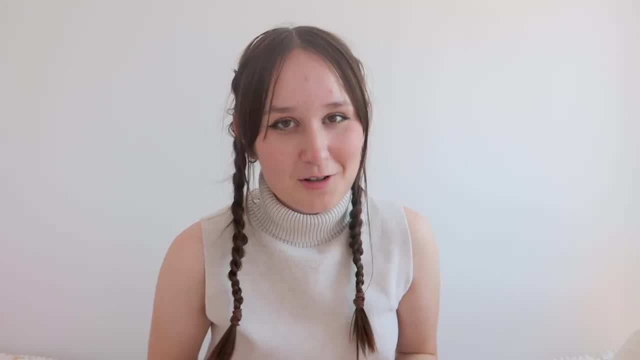 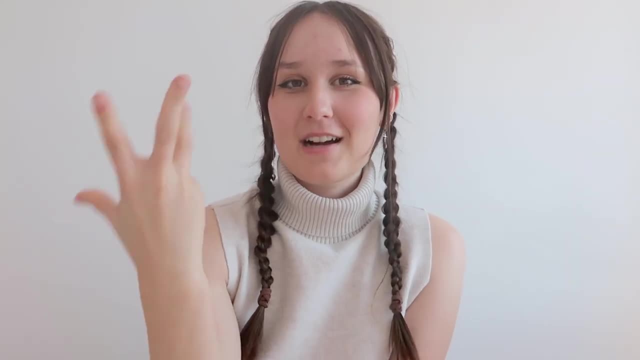 that's the one. last but not least, old greek god lovers are reincarnated as two students at a university during the modern day. this just seems fun to write. can you imagine like? just like like these star-crossed, like greek gods, just like reincarnated as immortals, but like in the modern? 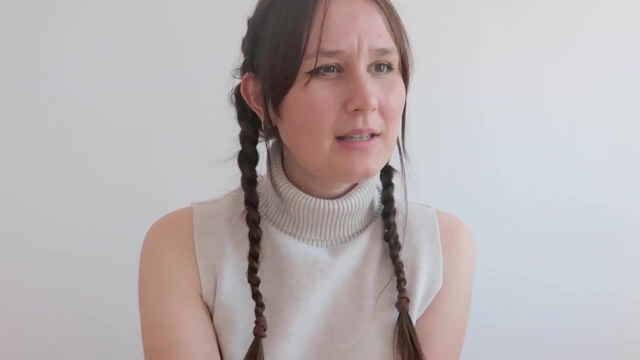 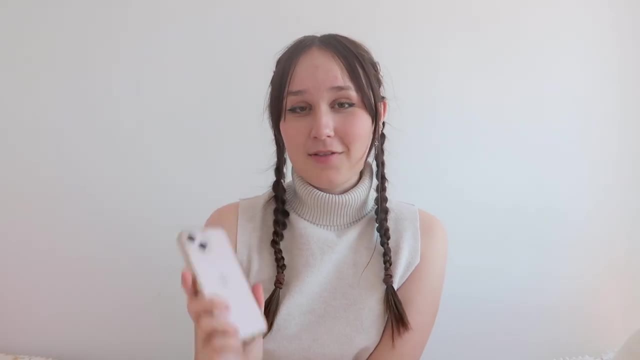 day with like cell phones and stuff like that. how would they cope? how would they cope? anyways, that's all the questions. i have not questions, sorry- all the ideas i have for this video. if you guys want more, i can definitely do a part three. this is part two, by the way. go check.